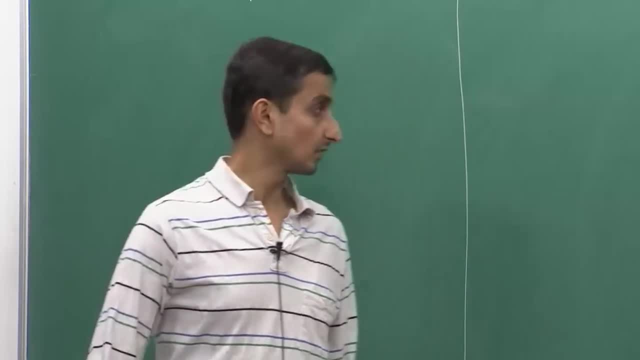 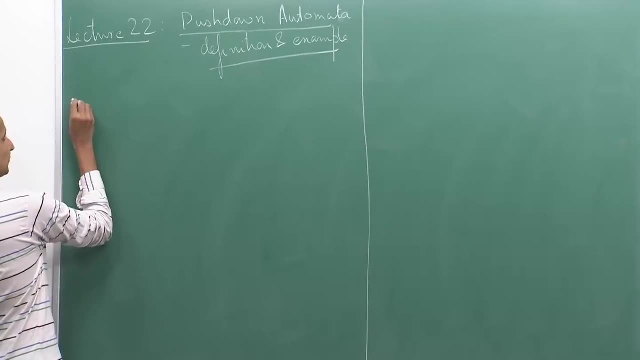 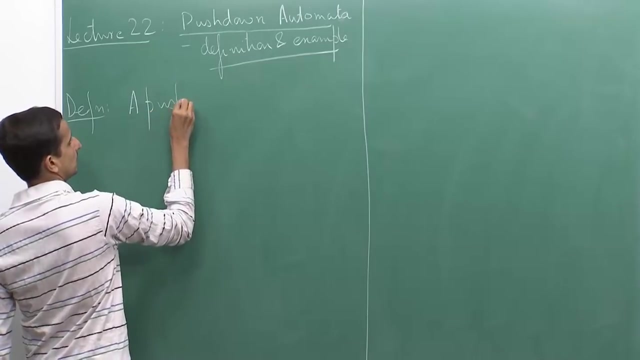 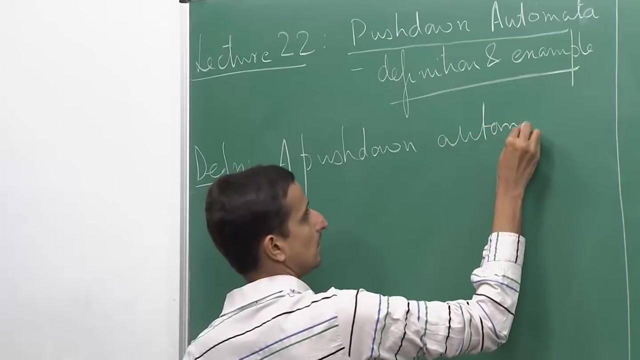 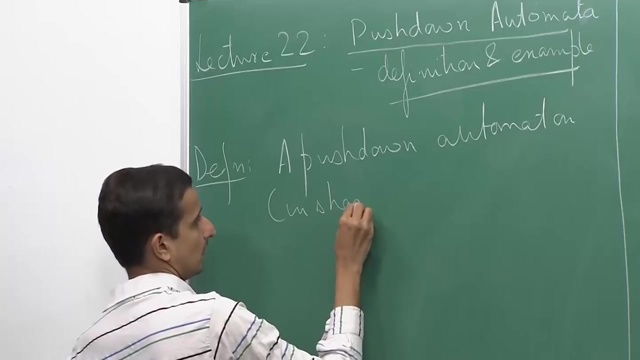 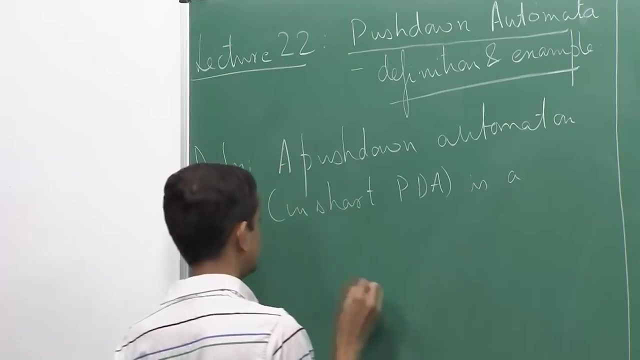 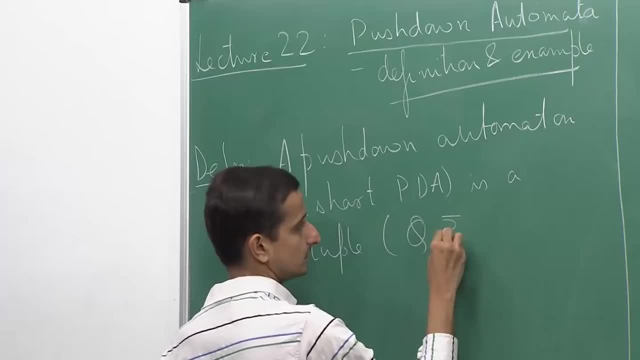 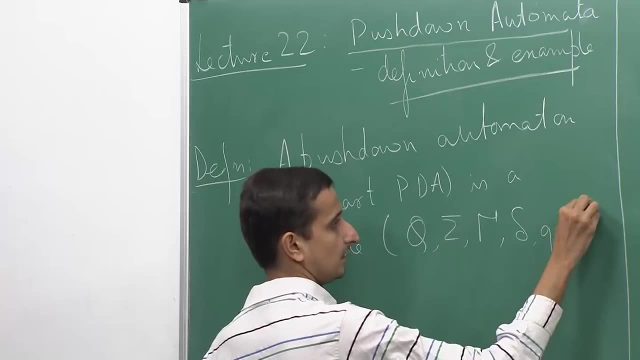 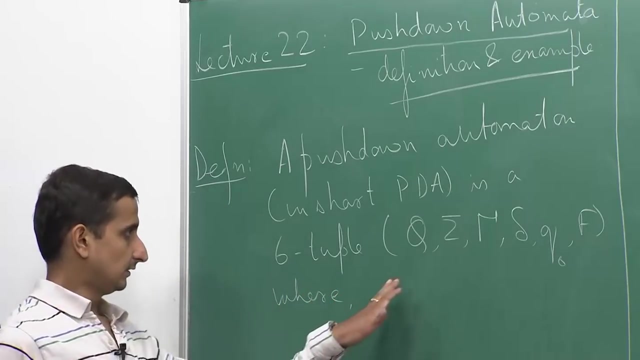 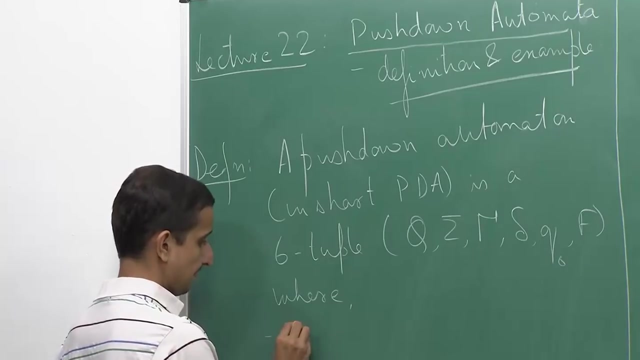 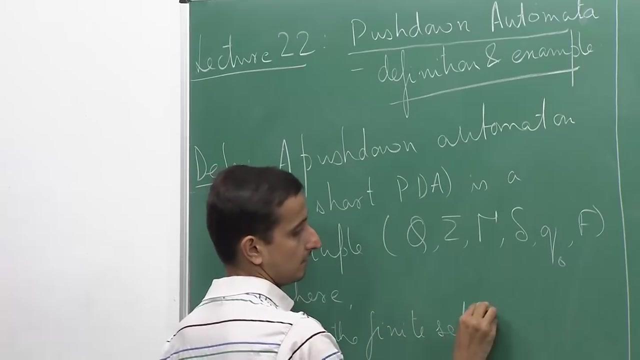 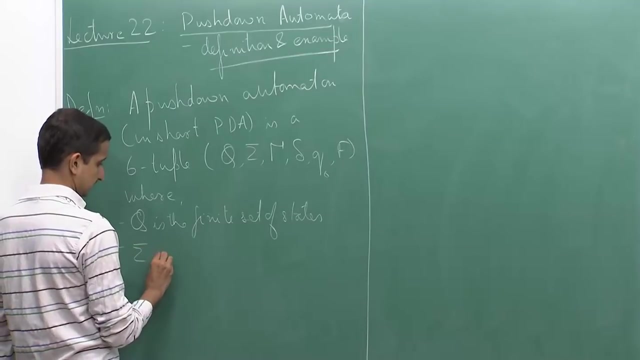 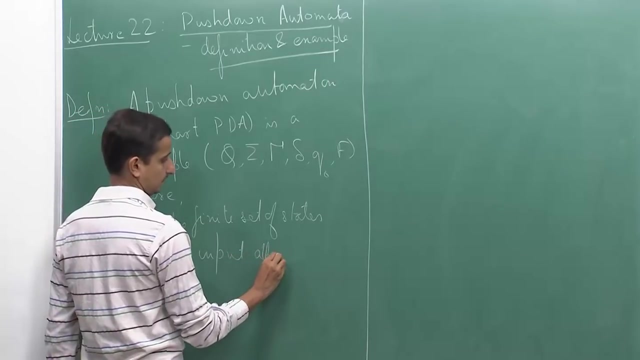 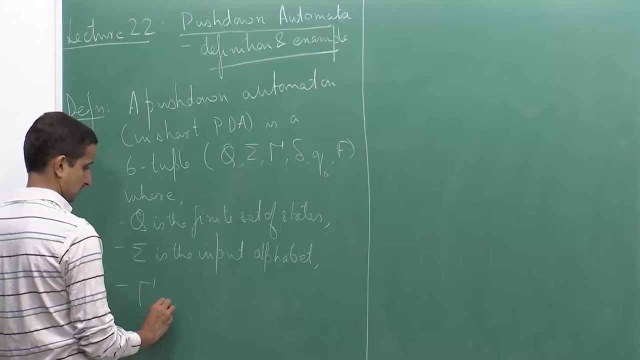 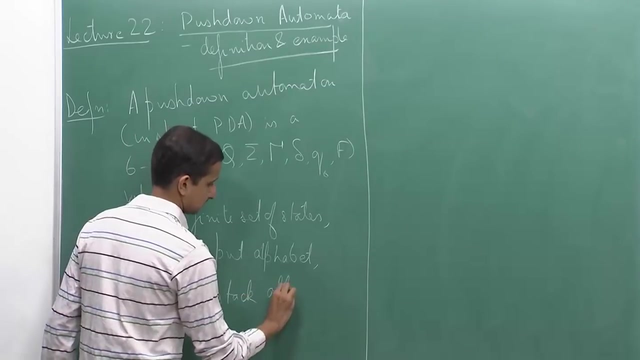 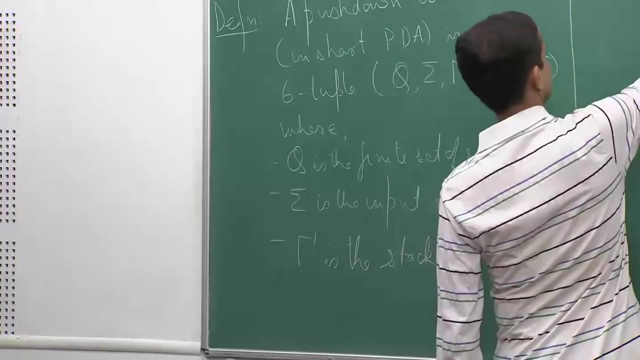 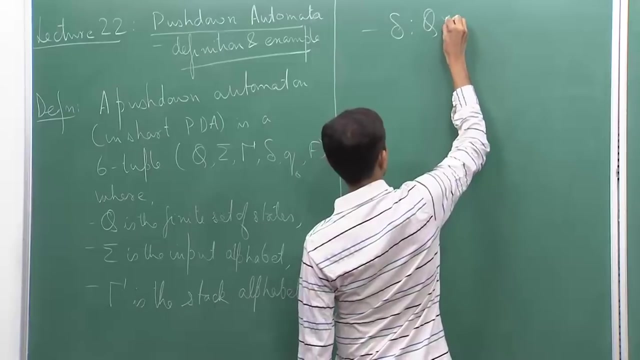 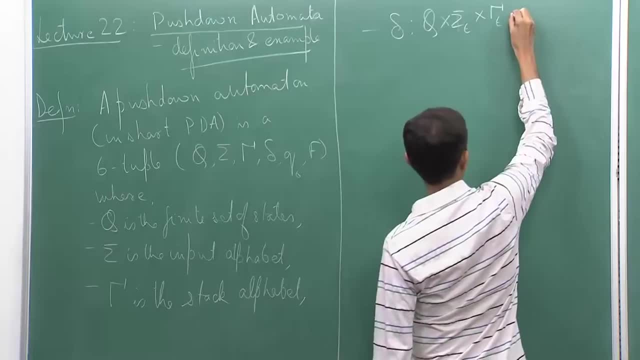 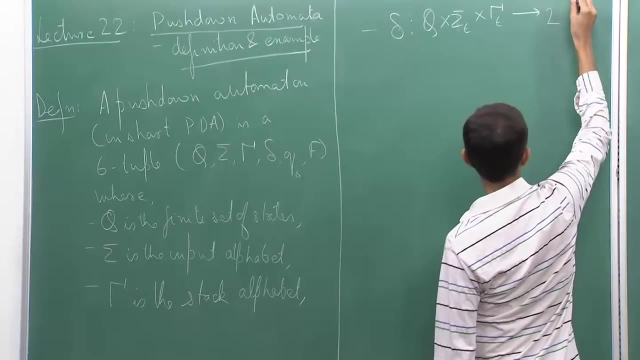 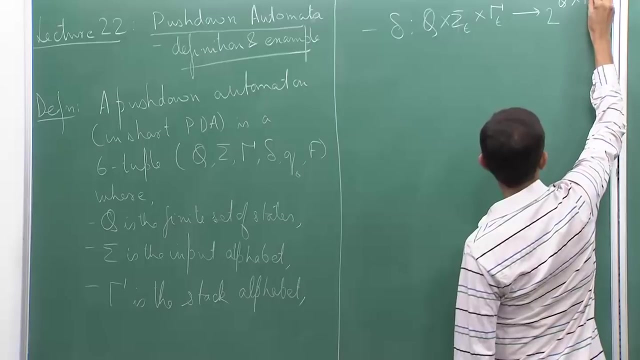 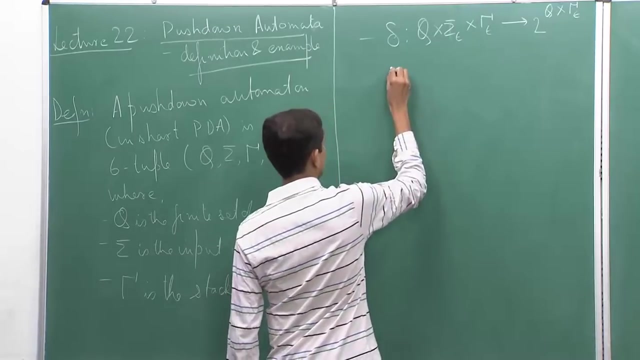 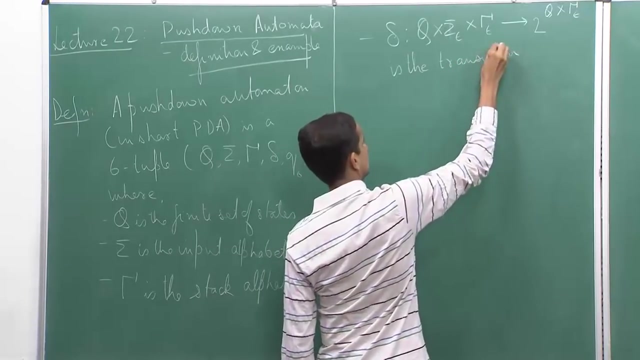 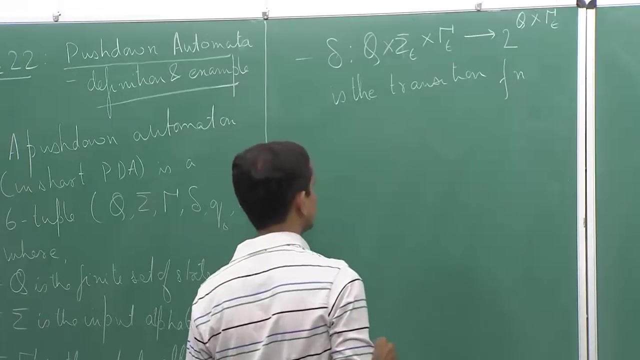 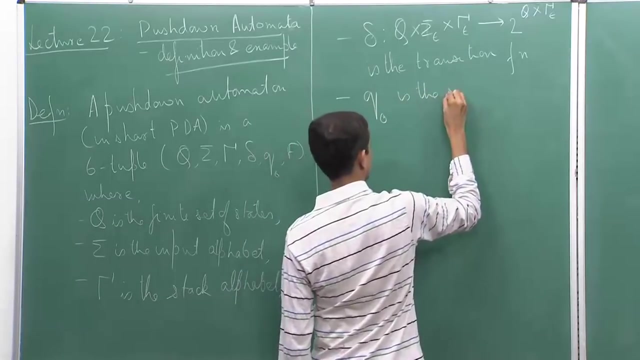 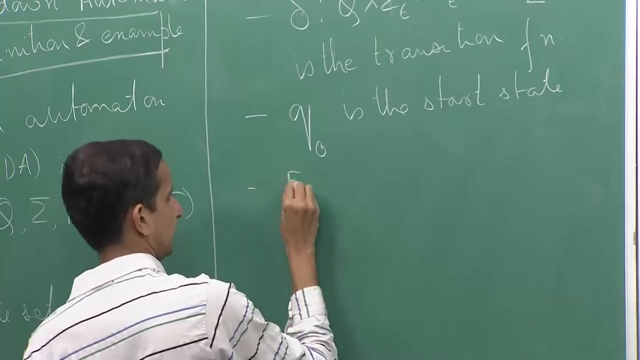 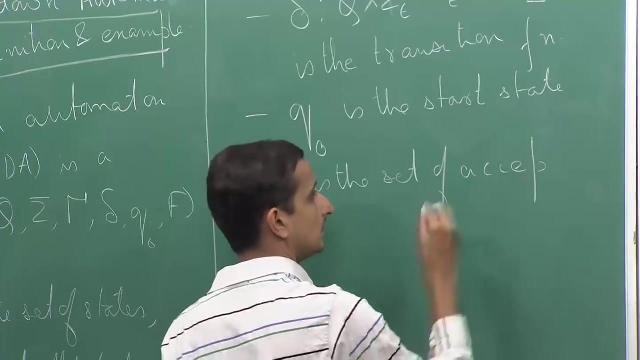 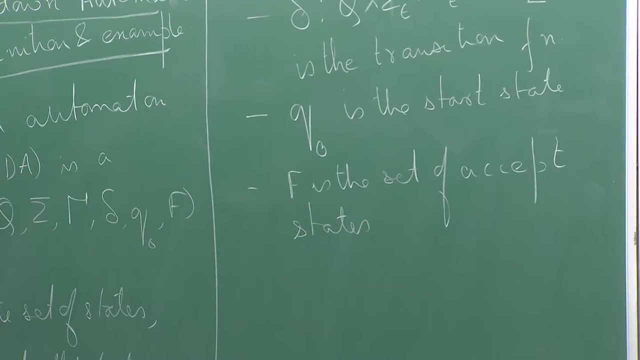 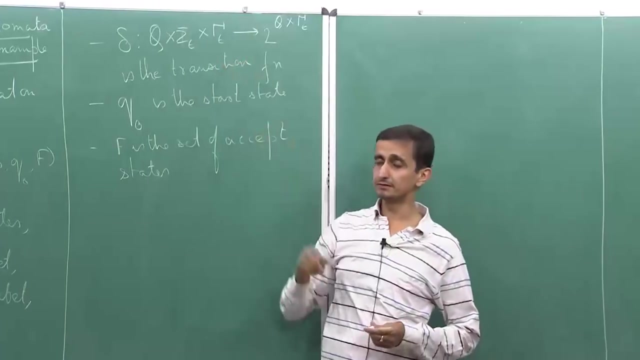 gamma epsilon to 2 to the power Q cross. gamma epsilon is the Transition function, Q naught is the start state and f is the set of accept states. So let me talk a little bit about the transition function, because 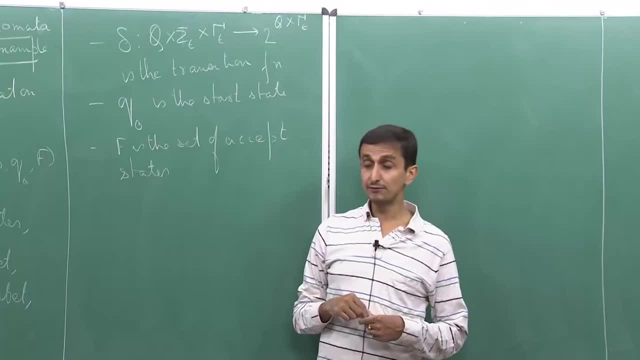 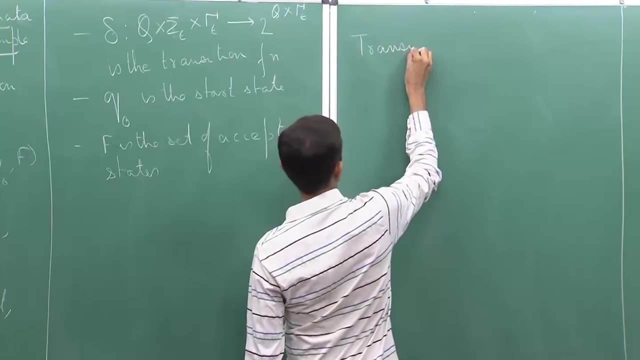 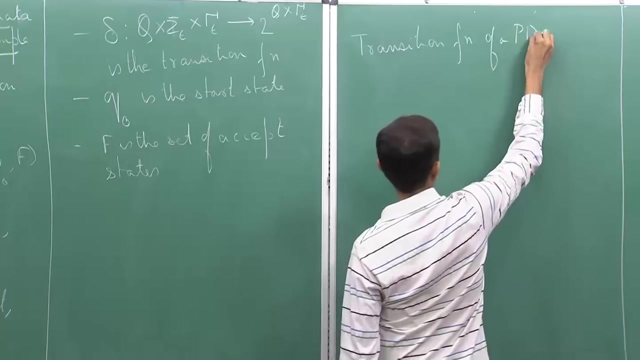 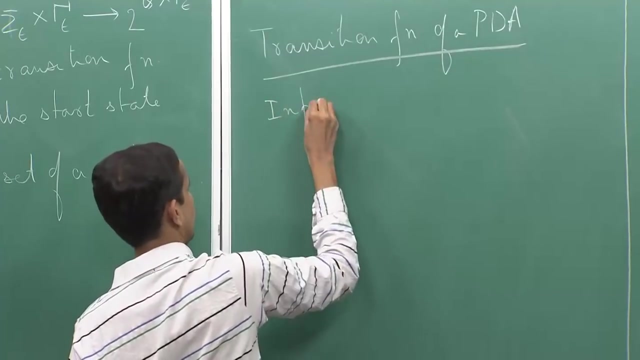 that is the thing which is different from that of a epsilon NFA. So the transition function takes the following as input. So if you look at it firstly, it takes a state as input. So if you look at it firstly, it takes a state as input. So if you look at it firstly, 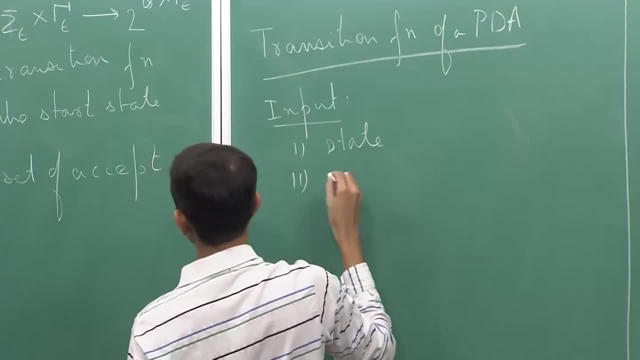 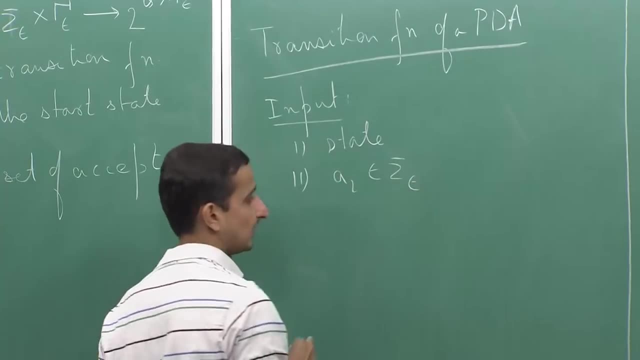 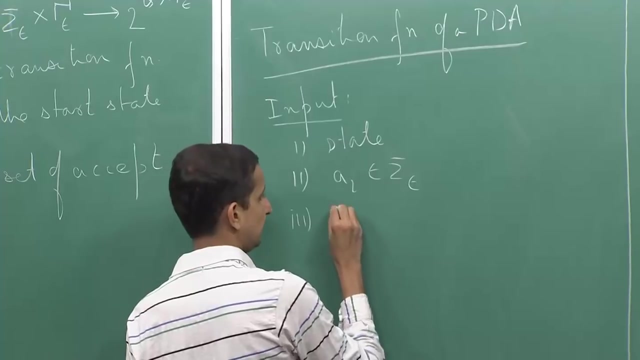 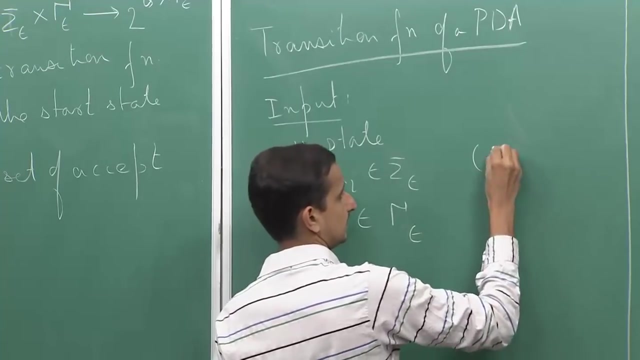 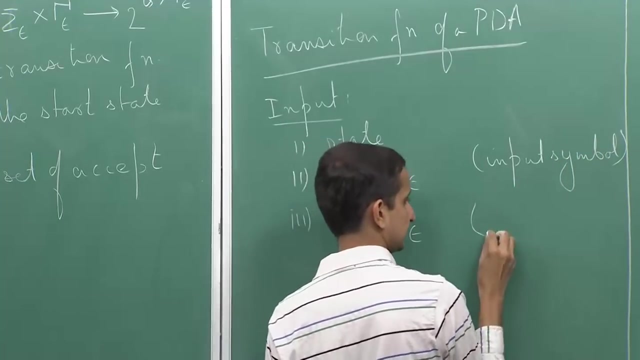 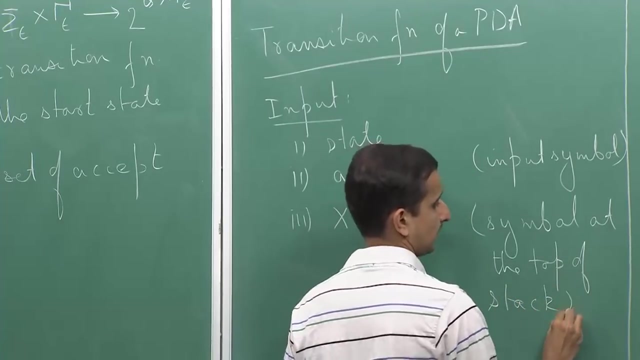 it takes a state as input. It takes a symbol ai in sigma epsilon as an input. So basically, this is the input symbol and it is reading a symbol x in gamma epsilon. So this is input symbol and this is symbol at the top of the stack. So it is taking these things as input. 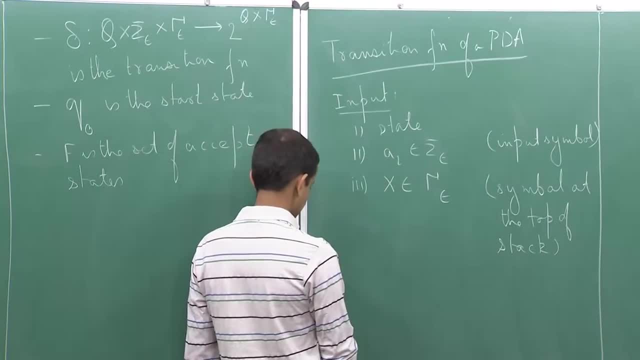 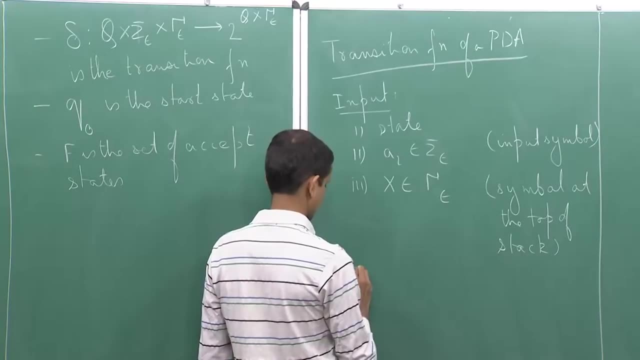 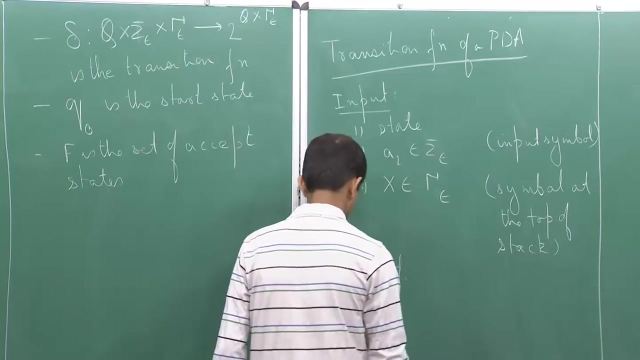 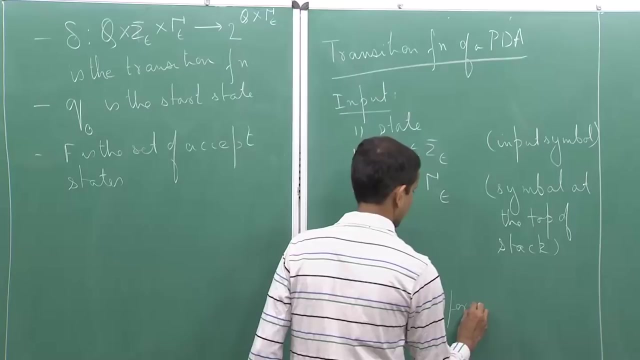 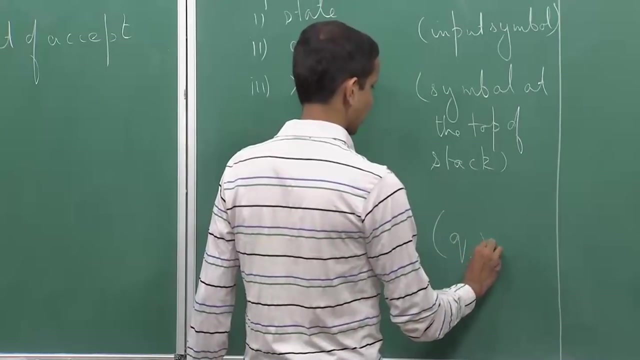 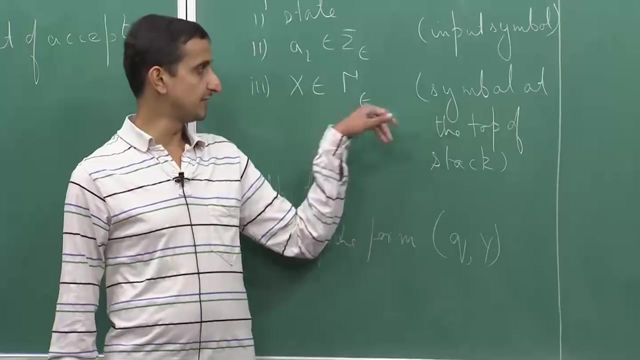 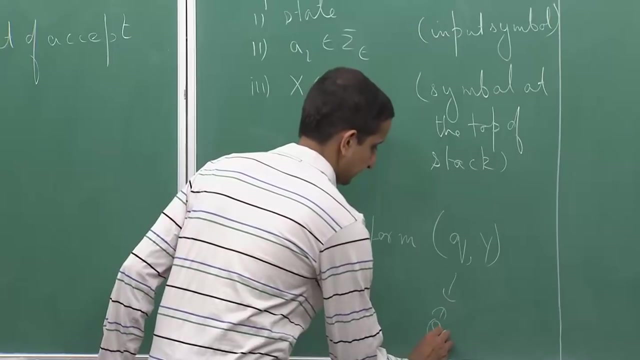 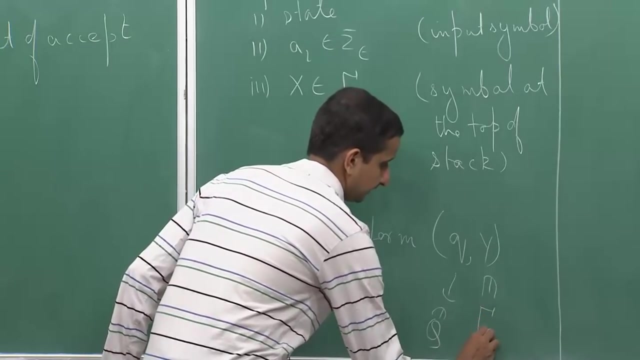 and what it is producing is. it is producing pairs of the form, So some q comma y, where q is the new state that you go to and y is the symbol with which you replace x. So this guy belongs to capital Q and this guy belongs to gamma epsilon. So 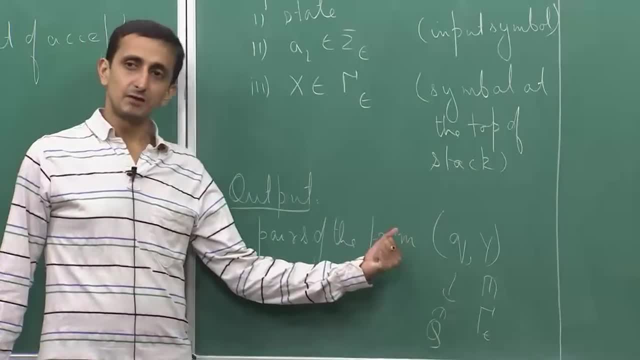 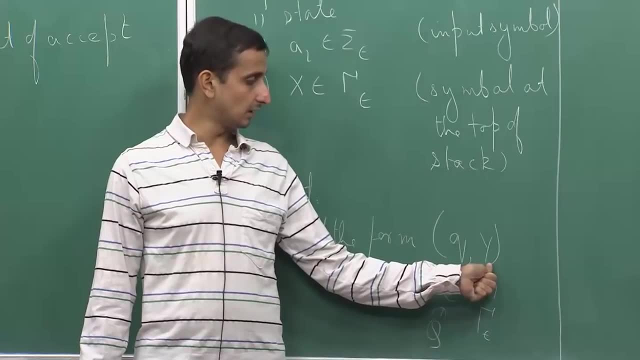 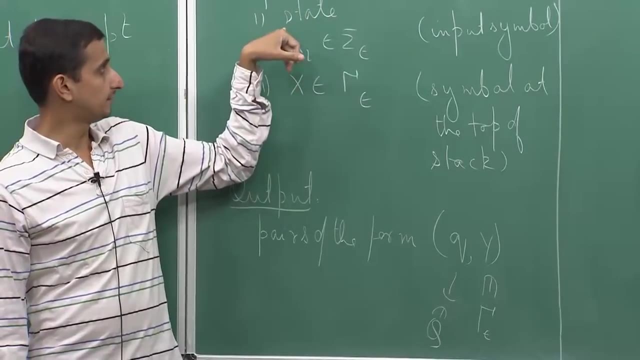 what do I mean by pairs? What do I mean when I say pairs? So it is not that it is just. it can output just one state comma: stack symbol pair. given a triplet of the form. So let us say here the state is p, So given. let us say p a i. 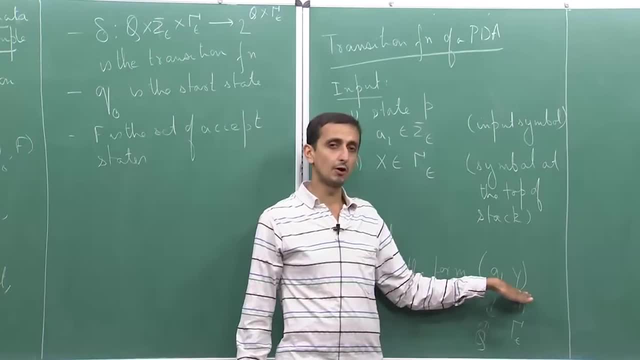 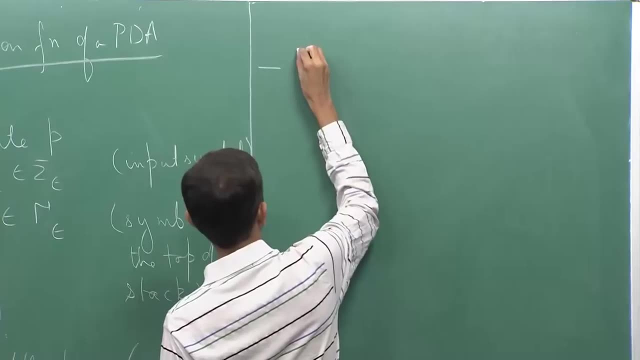 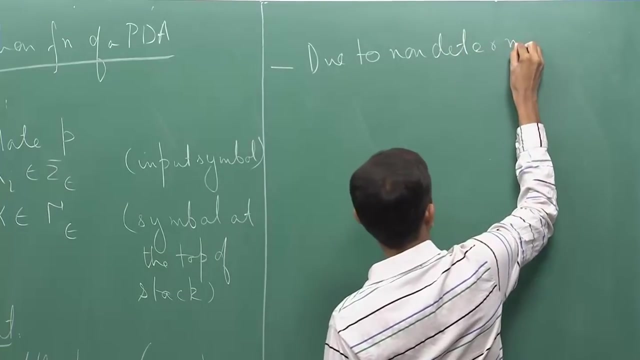 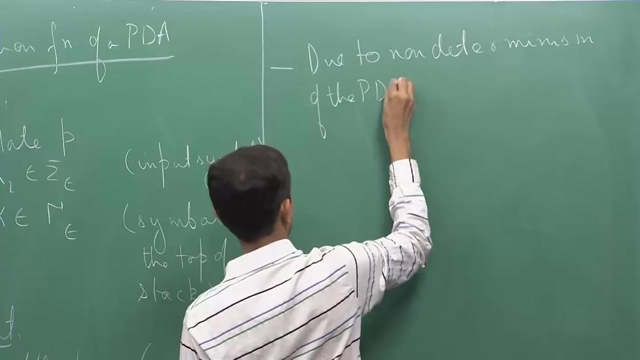 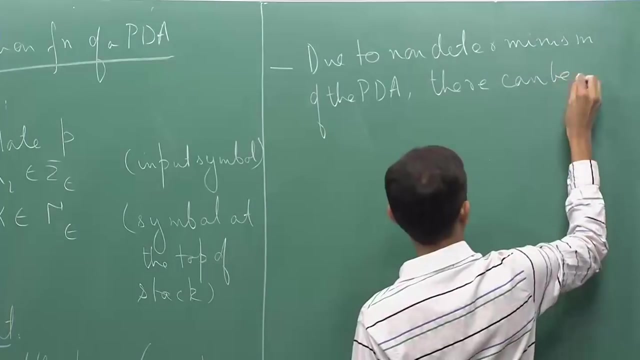 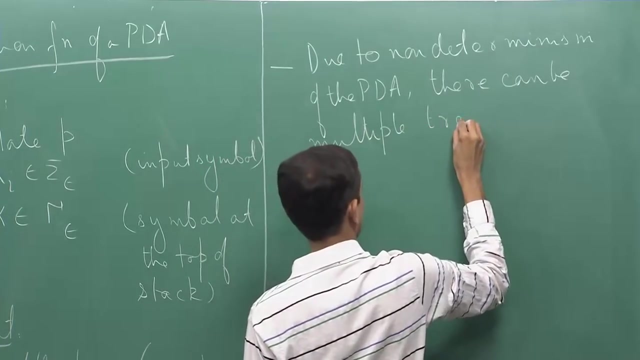 n, x, it can actually output multiple q, comma y. So this is because of the non-determinism, So So, So. so, due to non-determinism of the pushtown automator, there can be multiple items. 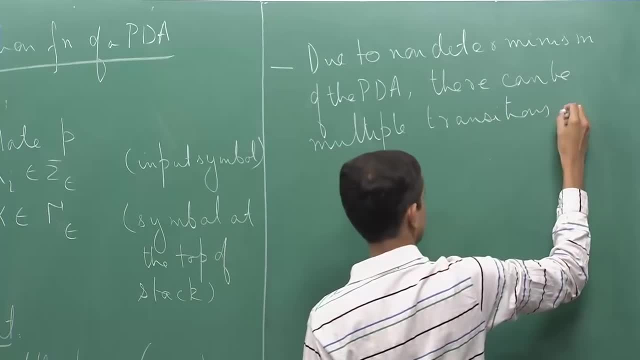 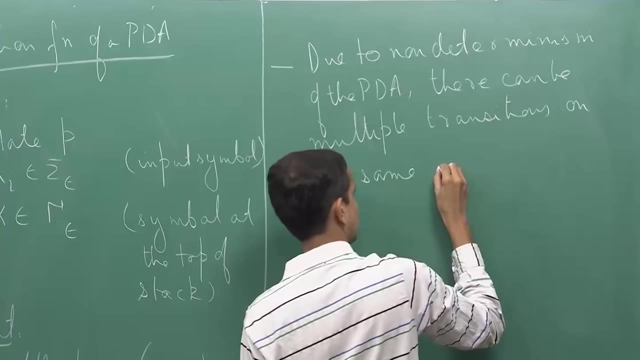 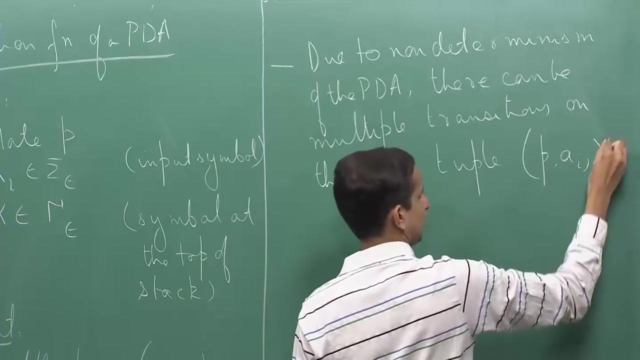 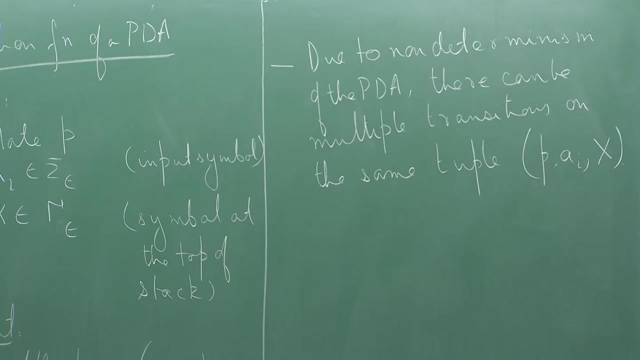 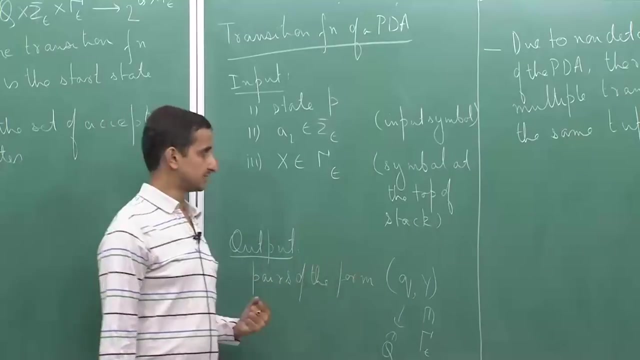 So transitions on the same tuple. let us say p, a, i and x. So this is where this is why we say that it is an epsilon NFA, a non-deterministic finite automata, because, as I said, that there can be multiple such pairs. 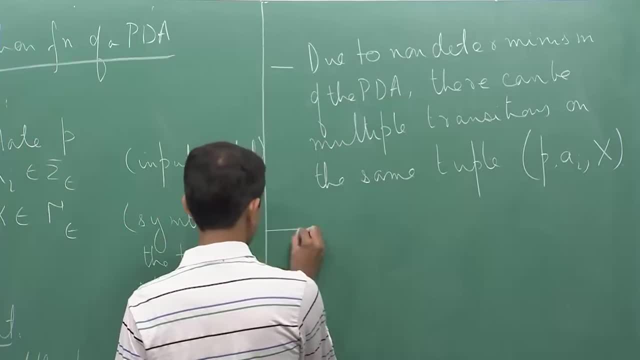 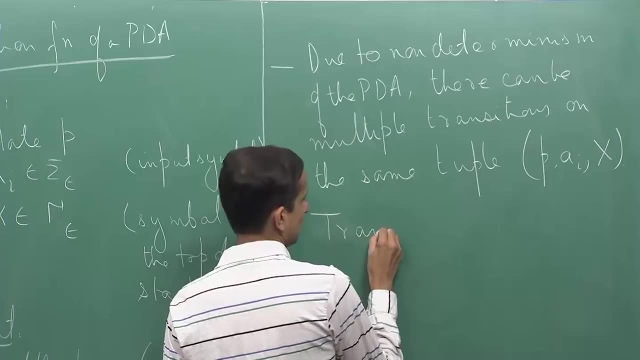 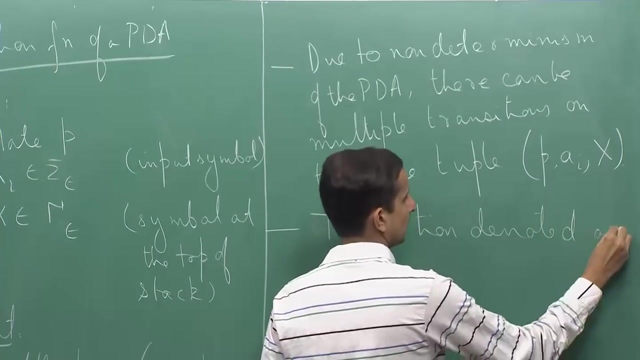 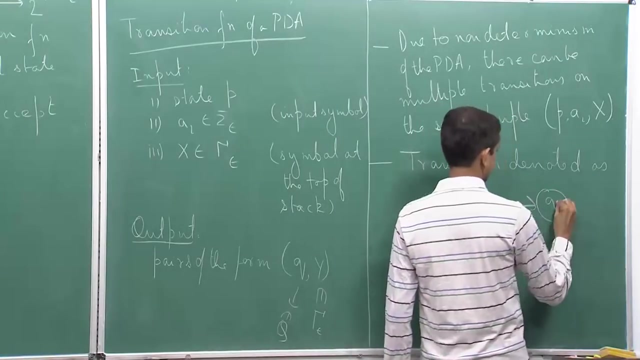 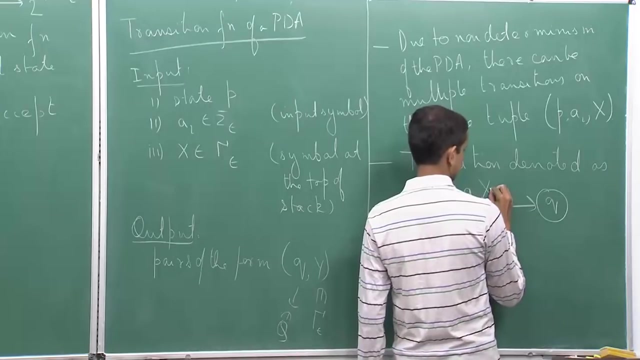 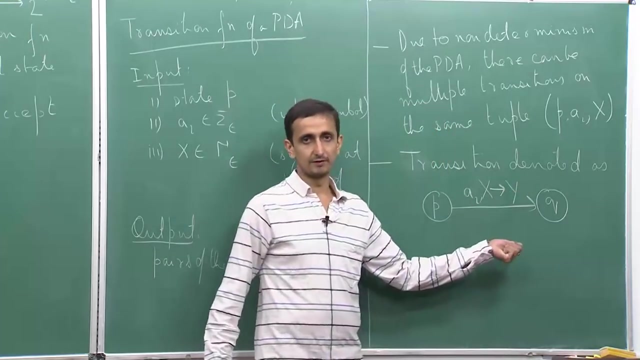 So this is this transition is denoted as, as from state p, you are going to some state q on reading the bit a- i and the stack symbol x gets replaced with y. So this is how a transition is denoted. So in the case of finite automata, we had just from p to q on a symbol a- i, but now we have. 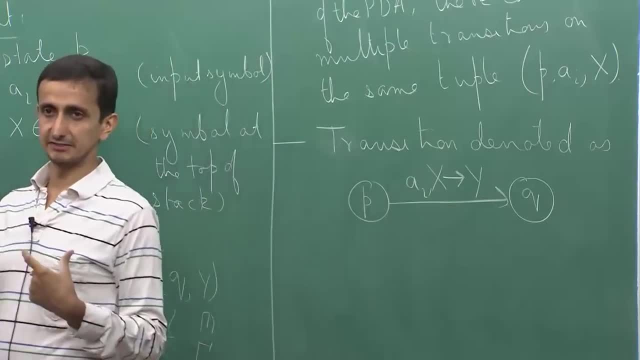 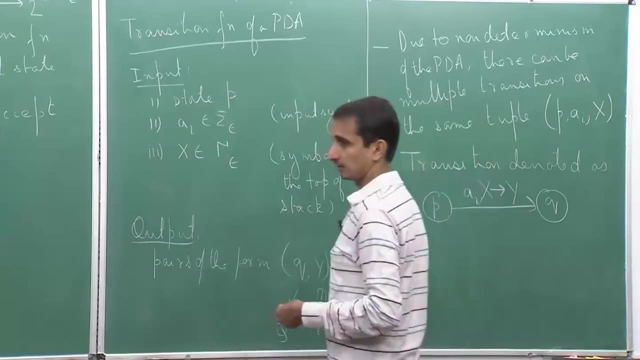 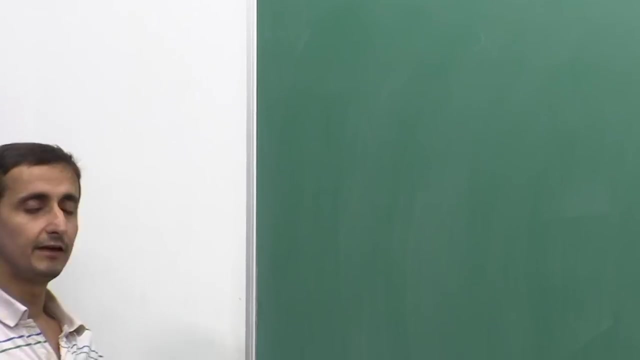 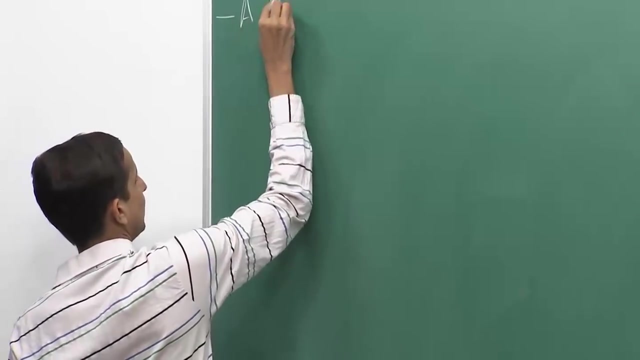 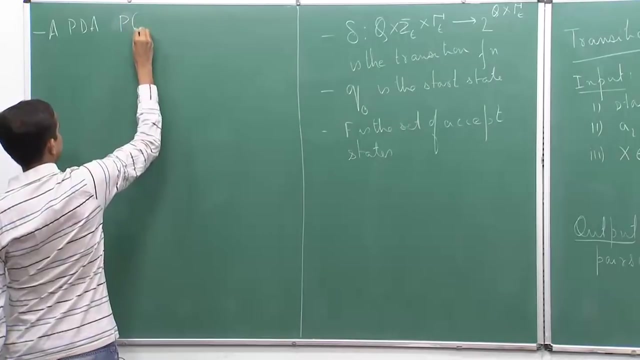 this additional thing to represent how the stack changes the behavior of the stack. So now let me define the computation of a push-down automata, So a pda, let us call it. p equals q sigma gamma p. Okay, Okay. 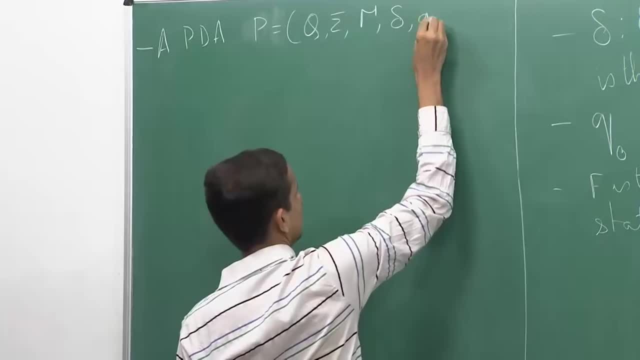 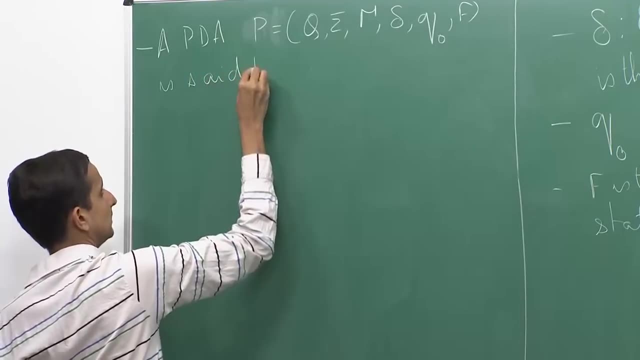 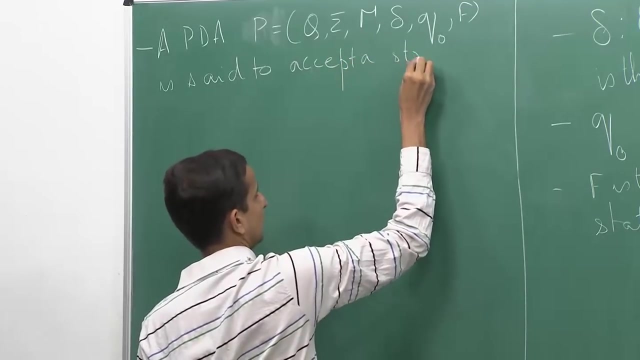 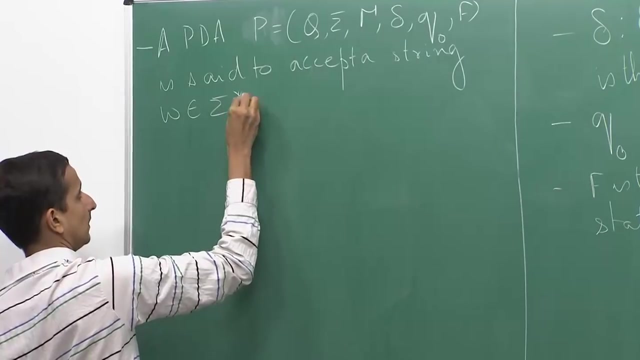 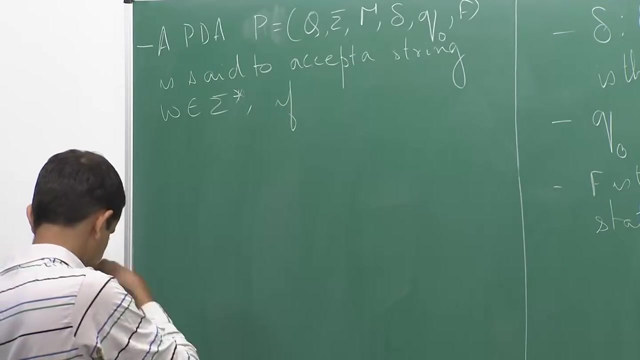 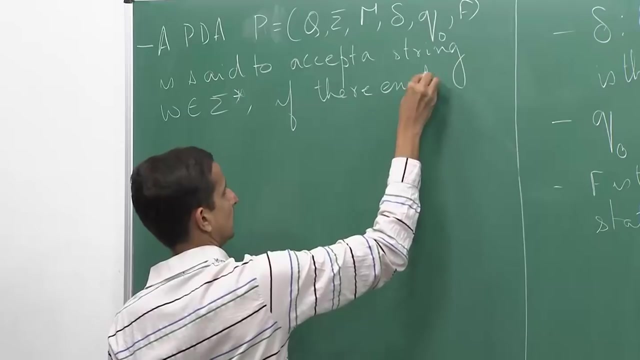 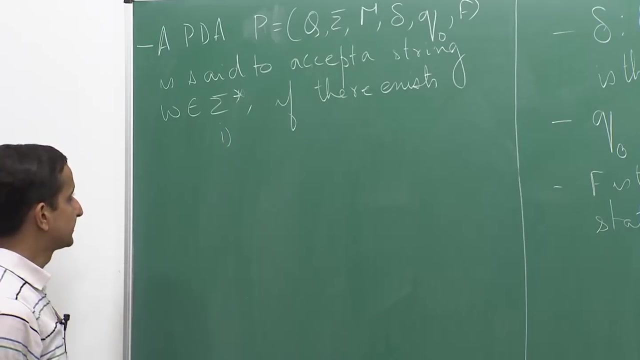 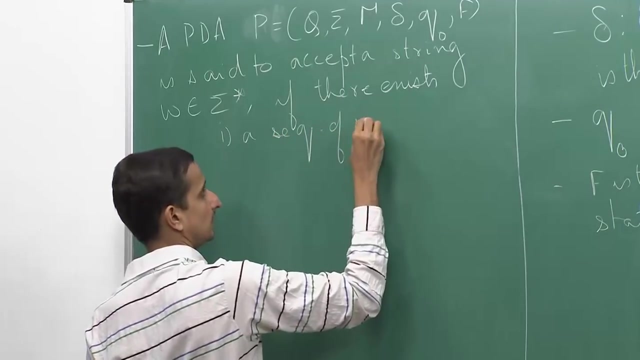 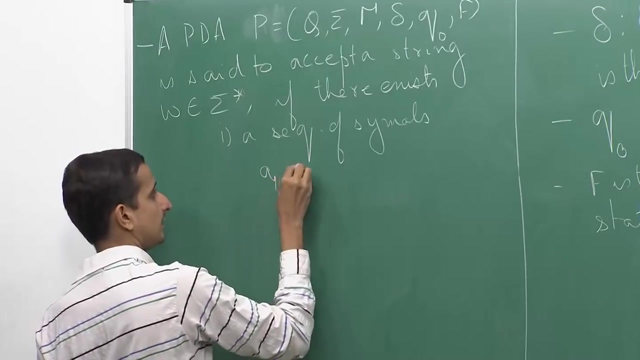 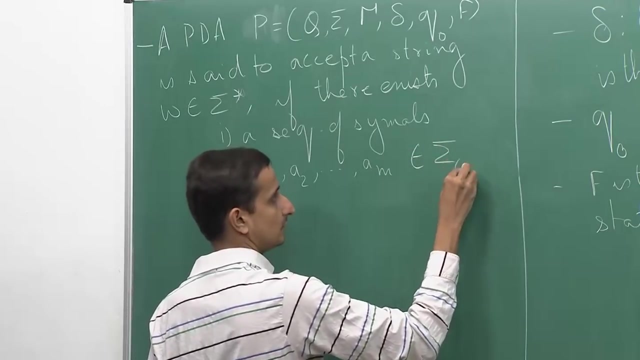 Okay, So pda, gamma delta u0 NF is said to accept a string w in sigma star. Okay, So there exists. so there exists three things. Firstly, there exists a sequence of symbols, Okay Okay, a 1, a 2 up to a m, each belonging to sigma epsilon. so there exist m symbols belonging. 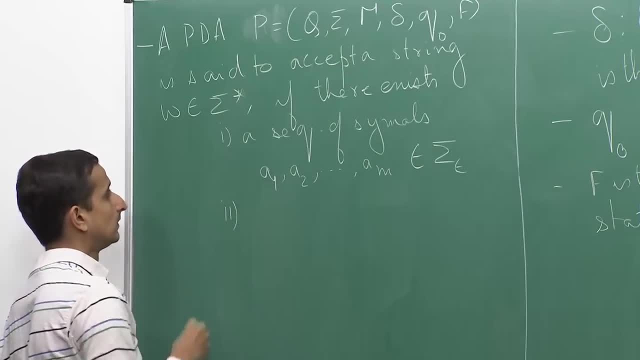 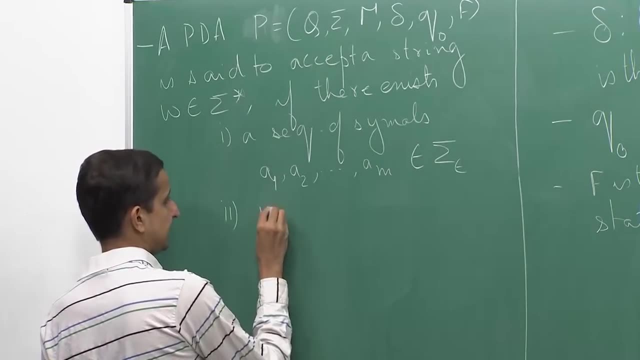 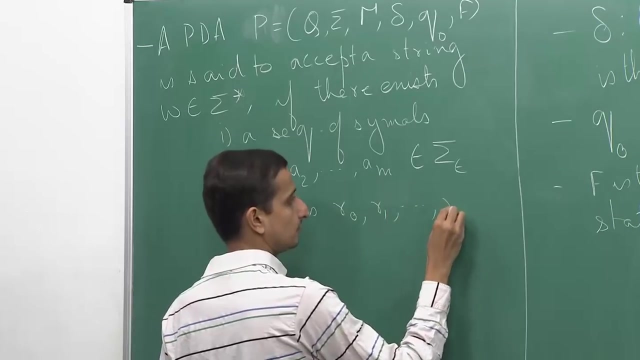 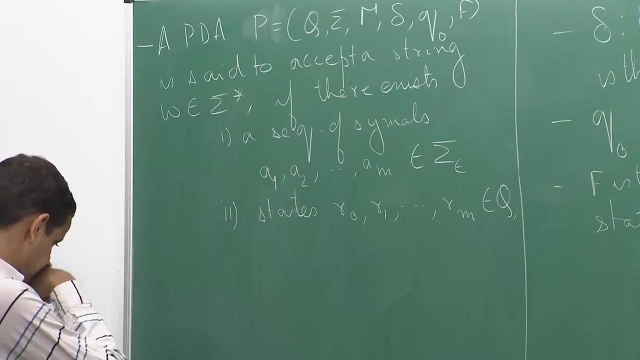 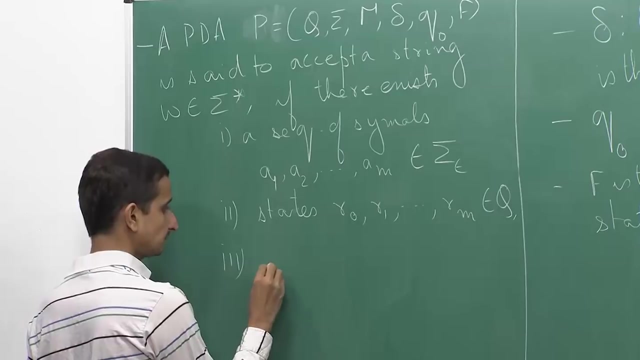 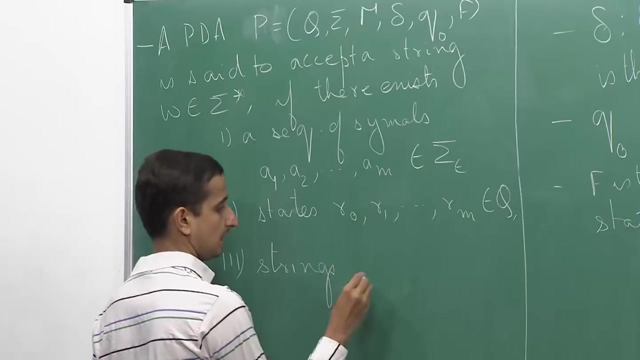 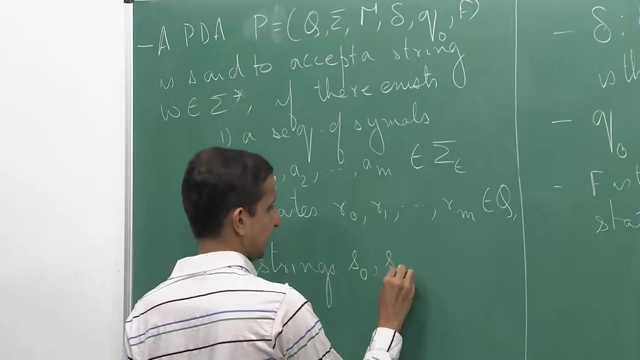 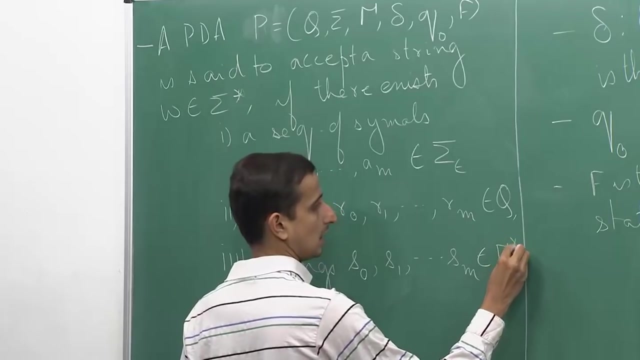 to sigma epsilon, there exist states r0, r1 through rm belonging to q and r0, r1 through rm belonging to q. So this is the first example. So we have strings S0, S1 up to Sm belonging to gamma star. so essentially, there are there. 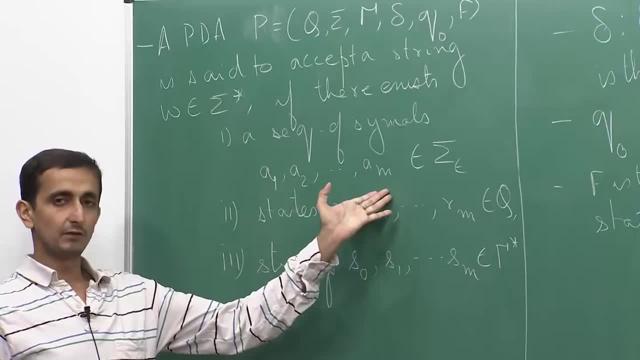 exist. so we assume three things: a1 through a2.. a2 through a3.. a4 through a5.. a6 through a6.. a7 through a8.. a9 through a10.. a11 through a11.. a12 through a12. 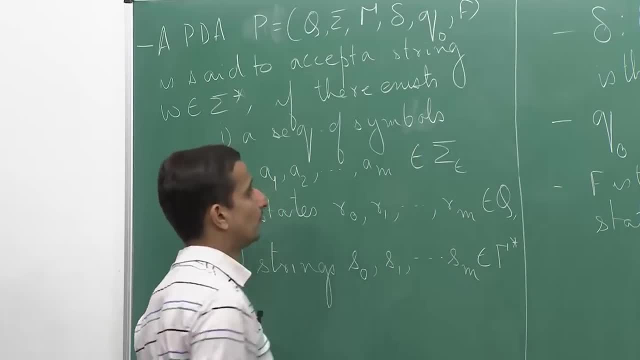 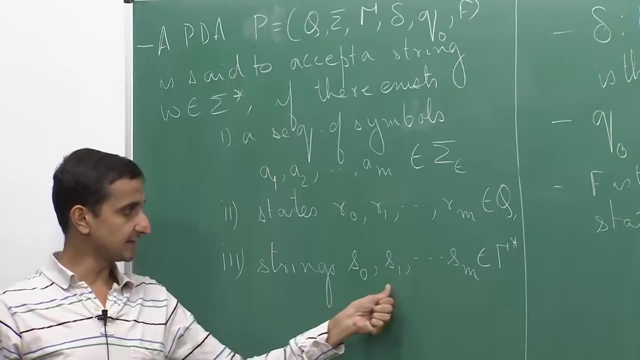 a13 through a13.. a13 through a13.. a14 through a13.. Which are symbols, from which are symbols in sigma epsilon. there exists states r0 to rm And there exist strings S0 through Sm over gamma star. so these are strings over the 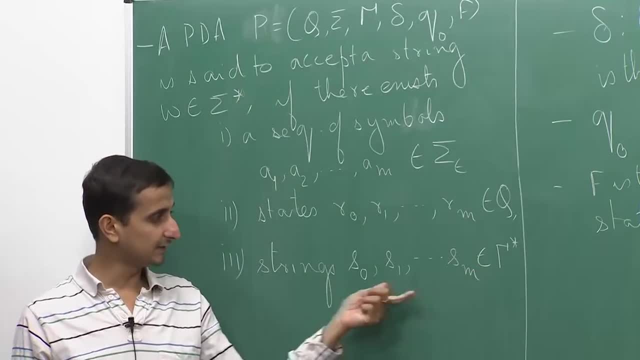 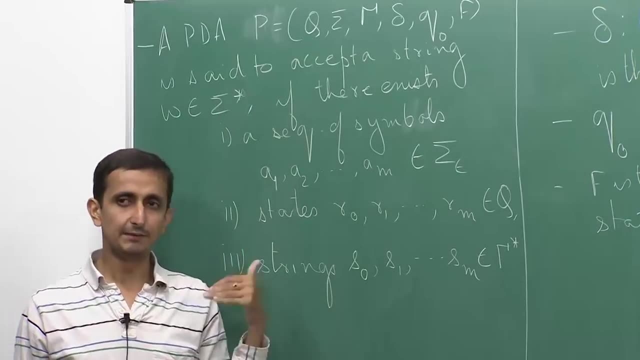 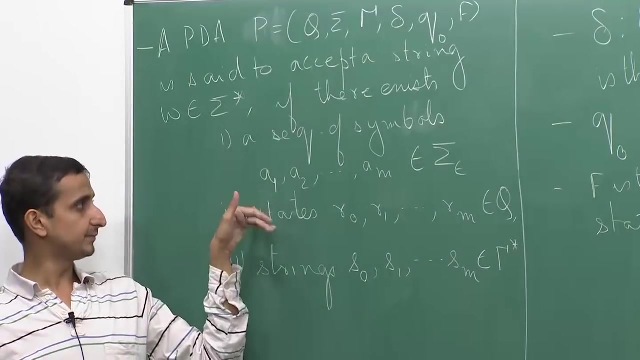 tape alphabet. So, essentially, intuitively, what these m states mean is that the PDA onметrics- I am sorry, Okay- when it receives the string w, it basically accepts a w in m steps, where, at each step, 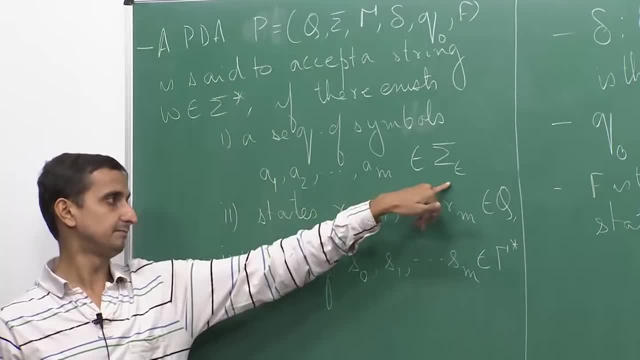 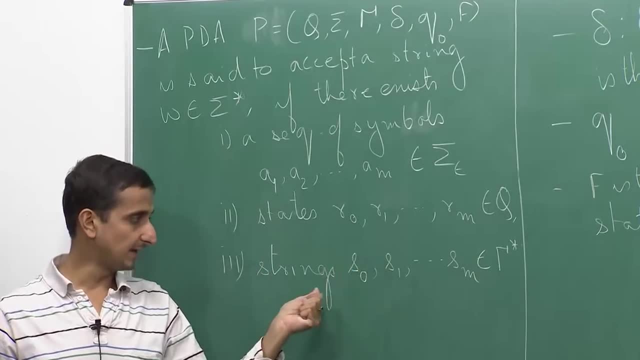 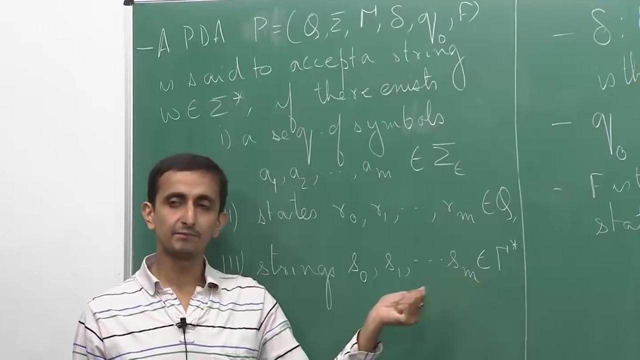 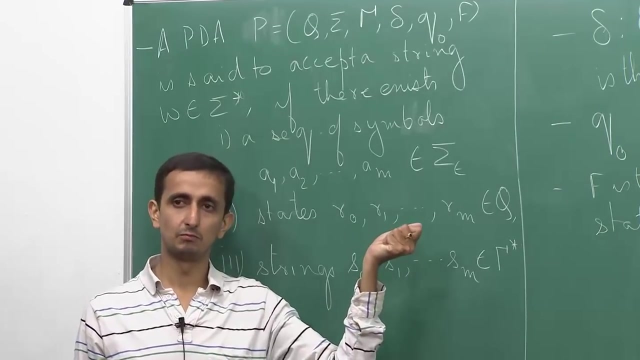 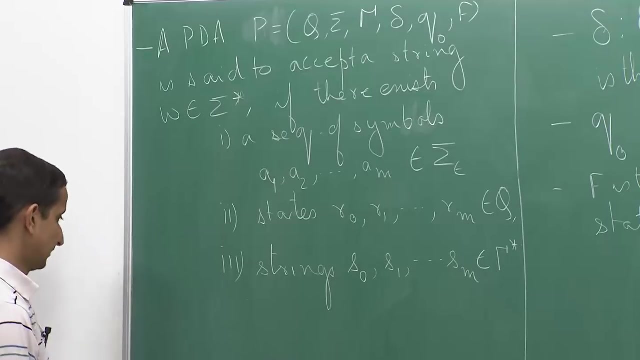 it is reading a i, So a i can be empty also. At each step it is going from a state r i minus 1 to r i, and at each step the contents of the stack is basically s? i. So whatever string that is contained in the stack from top to bottom is s? i. So let me. 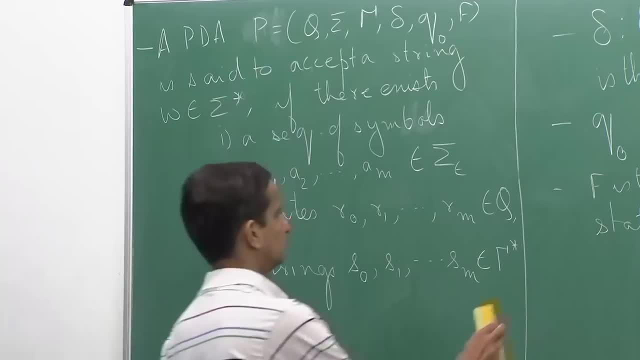 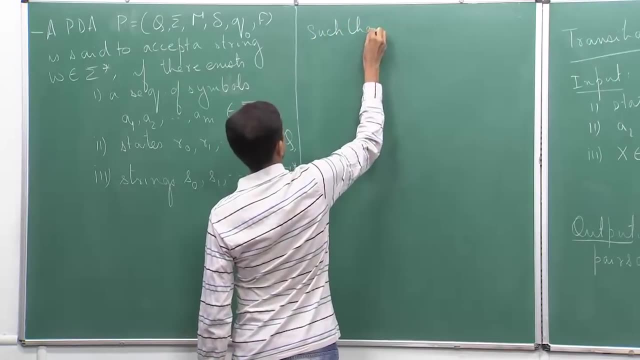 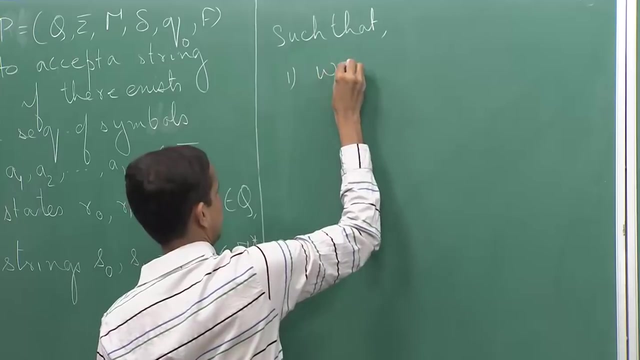 just rephrase what I just said such that, firstly, the string that is contained in the stack from top to bottom is s, i. So let me just rephrase what I just said such that, firstly, the string that is contained in the stack from top to bottom is w and w is 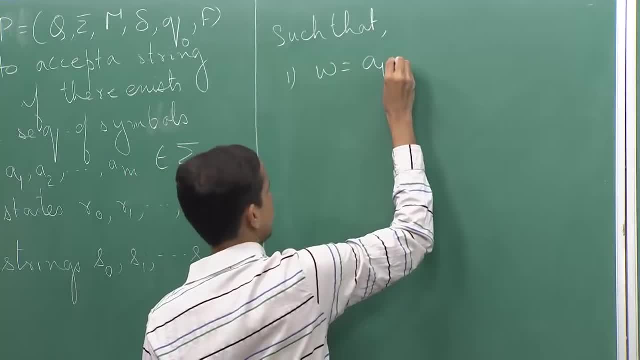 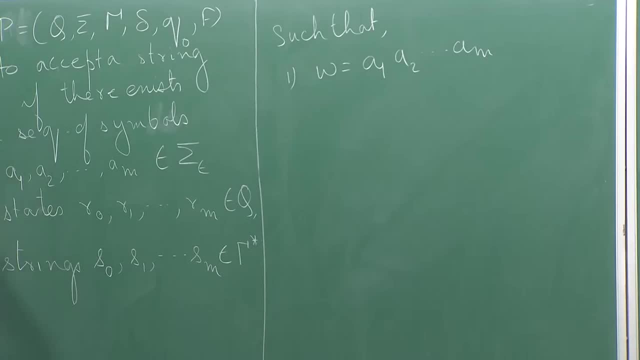 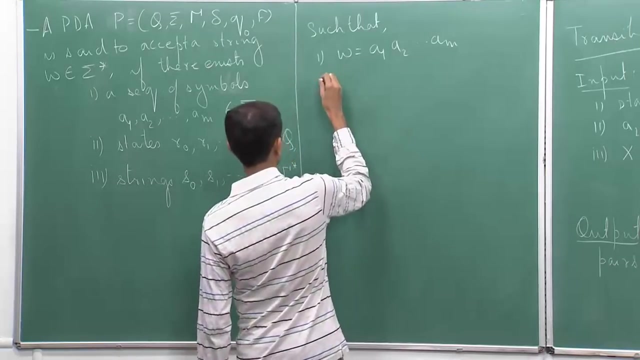 the string, the concatenation of the symbols a 1,, a 2 up to a m. So whatever input w that is given to us, it is nothing but the concatenation of the symbols that I read at each step. So 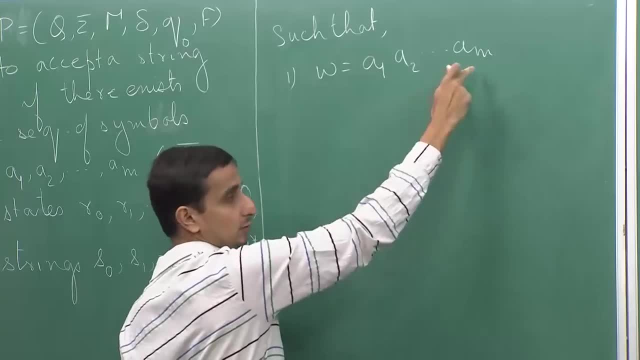 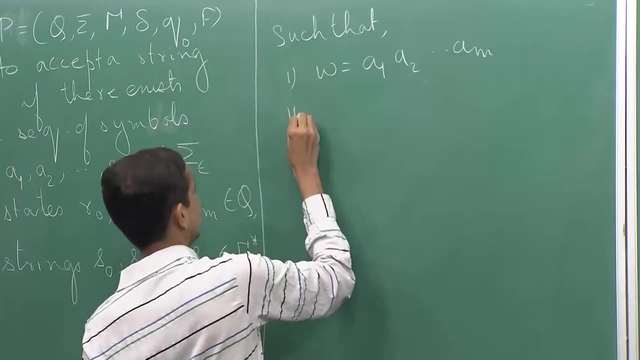 again note that some of these can be empty. So it is not that the length of w is m. The length of w is something that is less than or equal to m. Second is the initial condition. that is so what happens at the beginning. 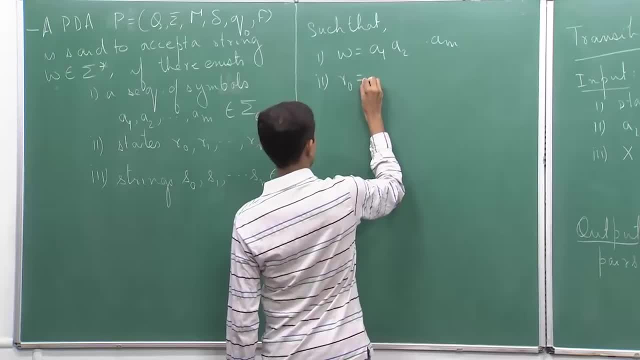 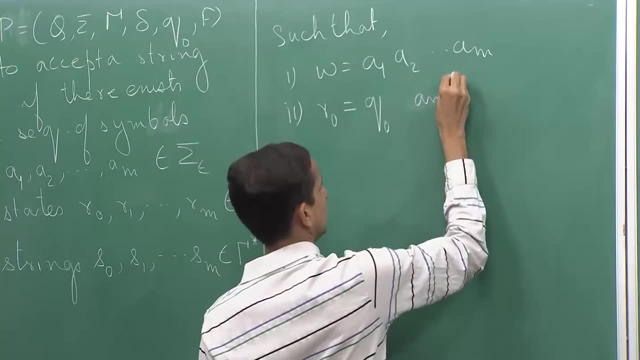 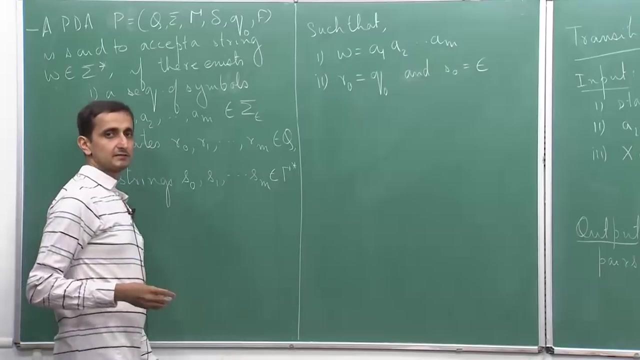 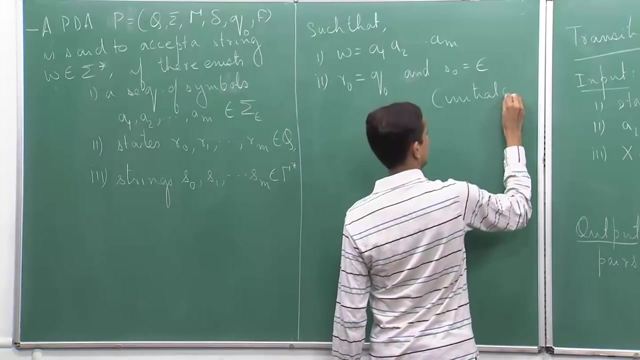 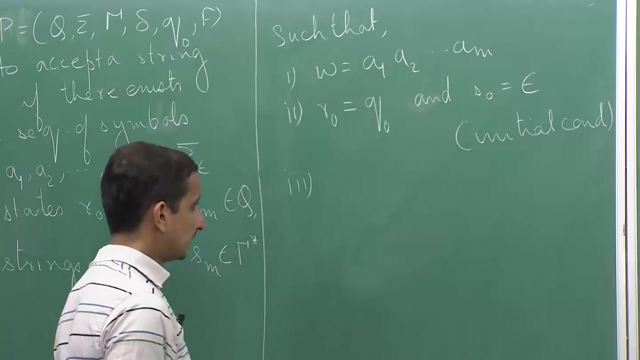 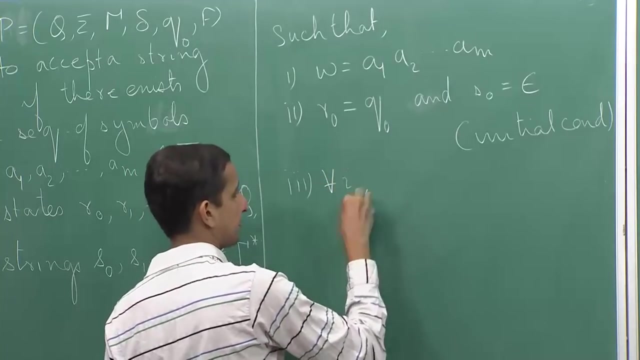 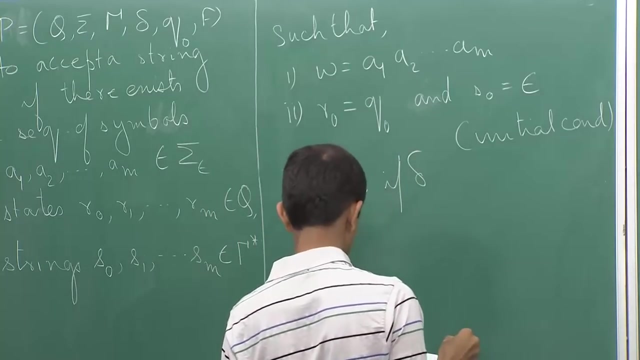 So at the beginning we have R0 equals Q0 and S0 is empty. So at the beginning the stack contains nothing. So this is the initial condition. Third is the transition condition. So we write the transition condition as for all i. what it does is: if delta is equal to 0, then the 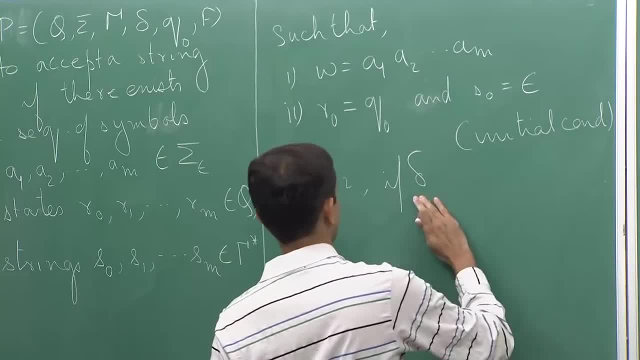 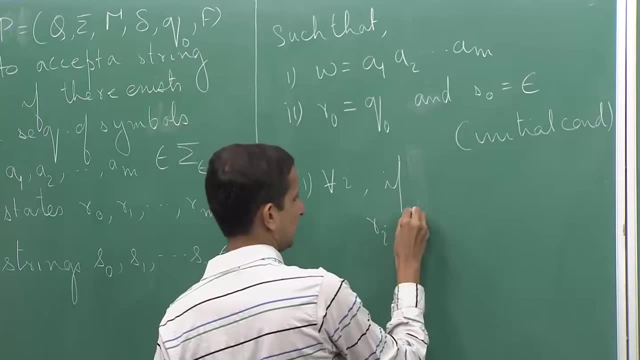 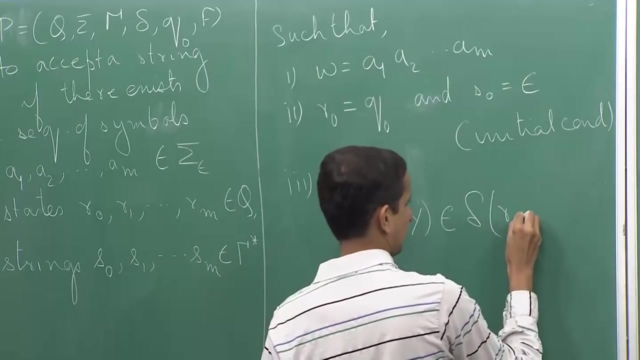 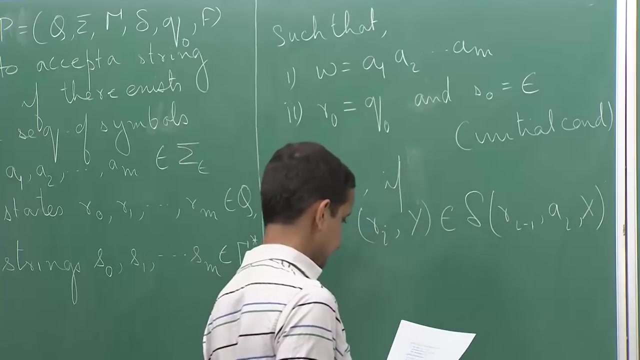 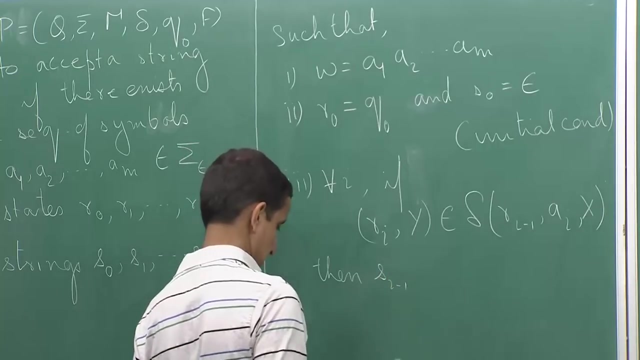 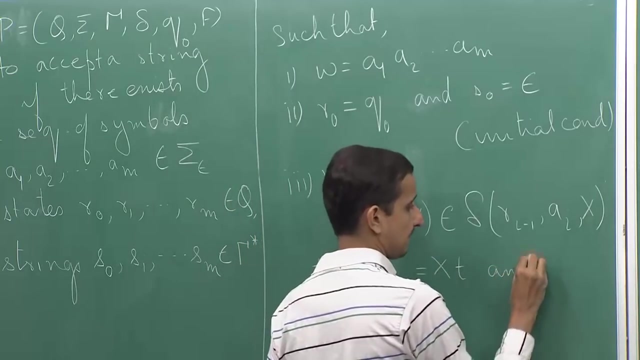 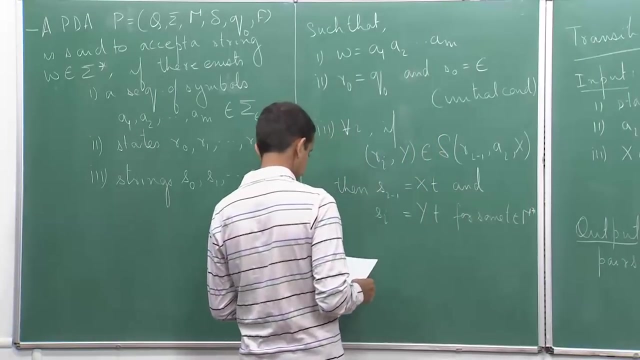 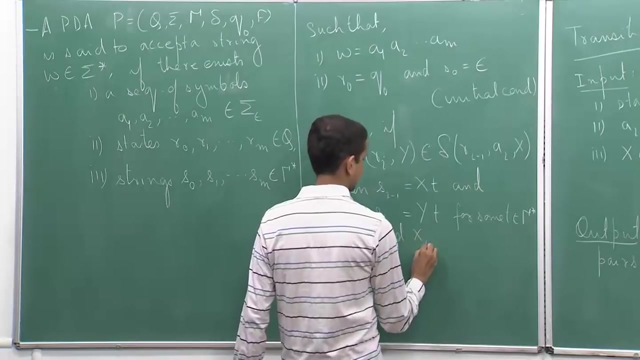 R0 is empty. If R is contained in delta R, A, X, then S is empty. So this is the initial condition. So at the beginning we have: R0 equals Q0 and S? i minus 1 is X, t and S? i is Y t- for some t in gamma star- and X- 1 is X. so this is A. 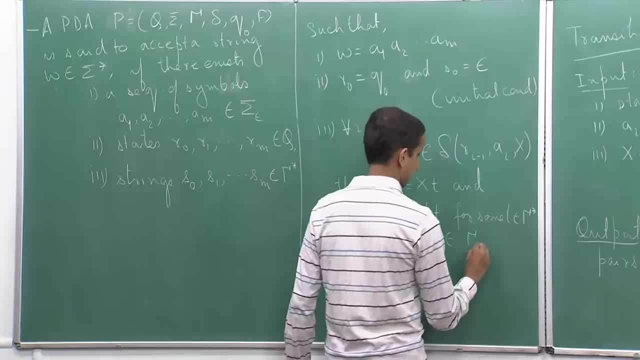 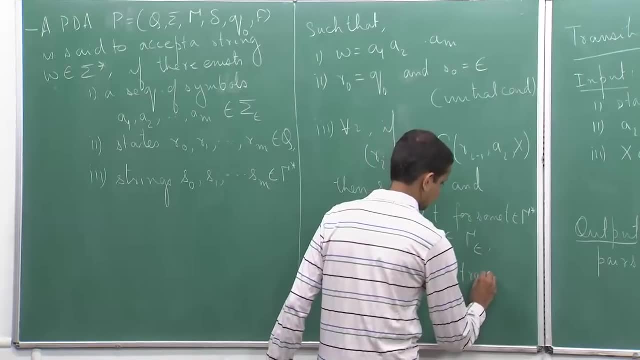 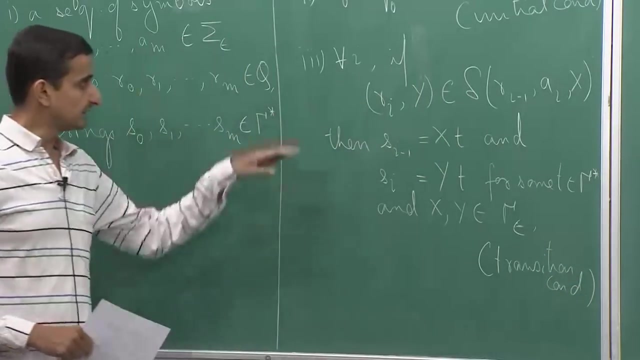 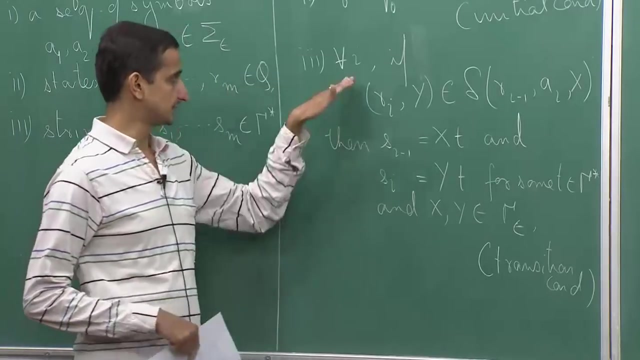 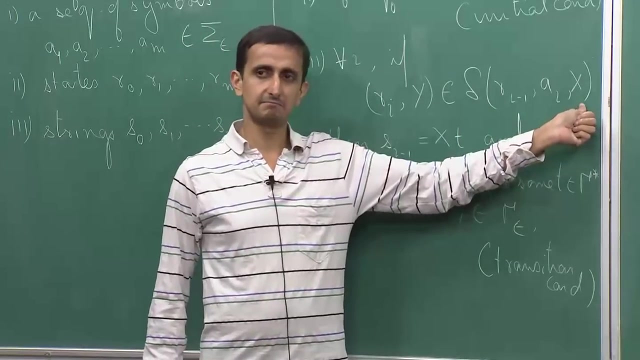 y in gamma epsilon. So this is the transition condition. So essentially what this is saying is that look at some i between 1 and m. So this is i in the set 1 through m. Now suppose if I look at delta, r, i minus 1, a, i and x, for some x, x can be any symbol in gamma epsilon. 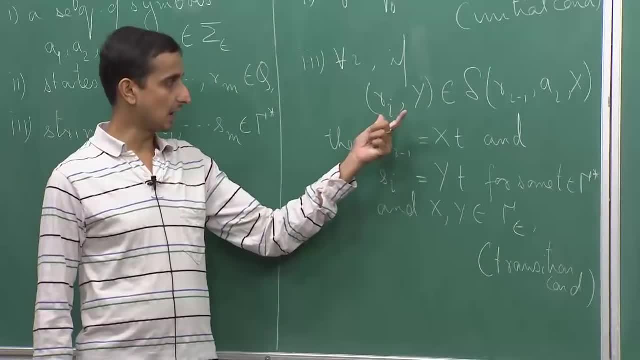 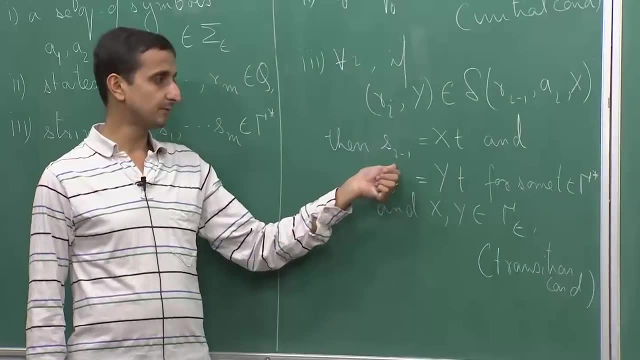 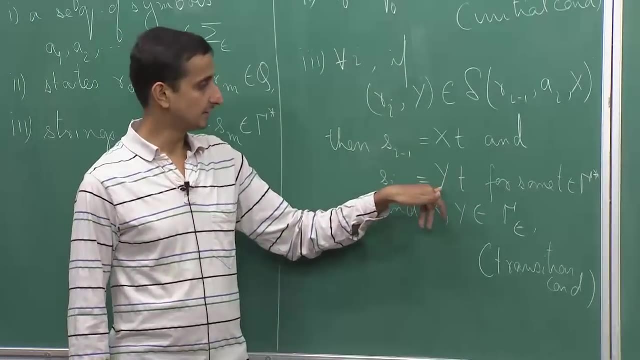 And if that set contains the pair r, i comma y, then the stack in the i minus 1th step should have had x at the top, followed by some string y, And in the ith step it got replaced that x got replaced with y. 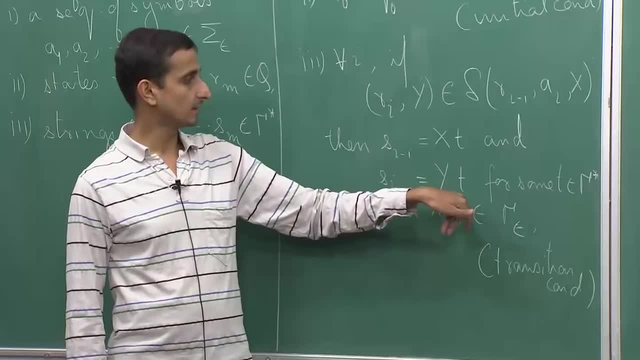 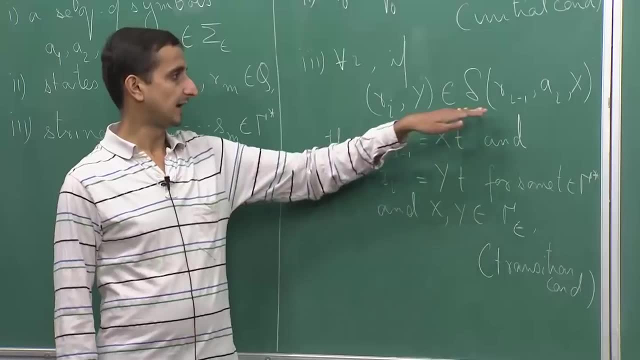 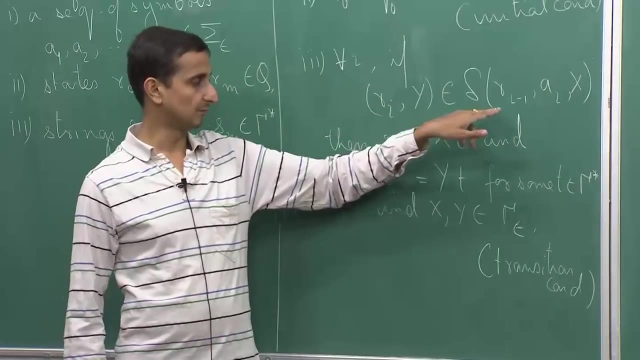 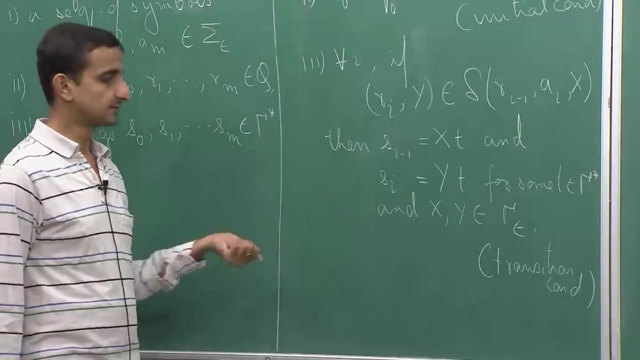 And the remainder of the stack remains the same. So it was t earlier, it remains t, And this essentially means that the computation moves from the r i minus 1, from the state r i minus 1 to the state r i. So this is what transition means, And when do we accept? 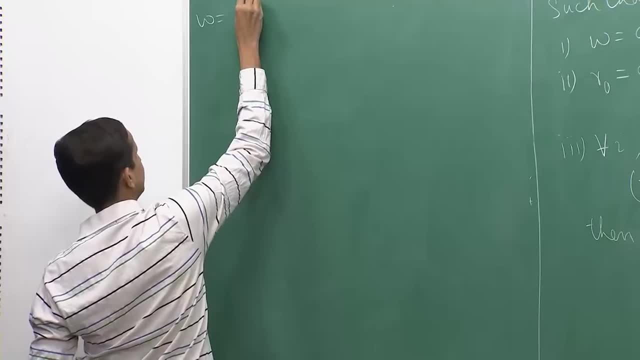 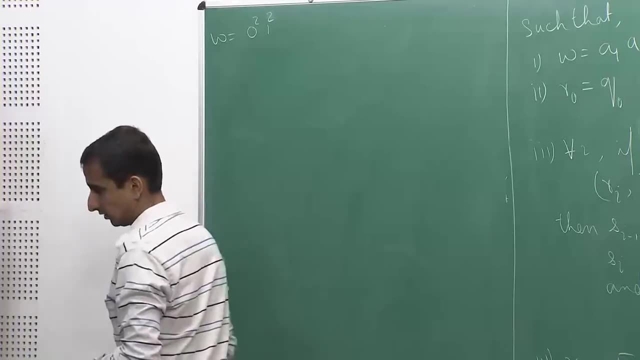 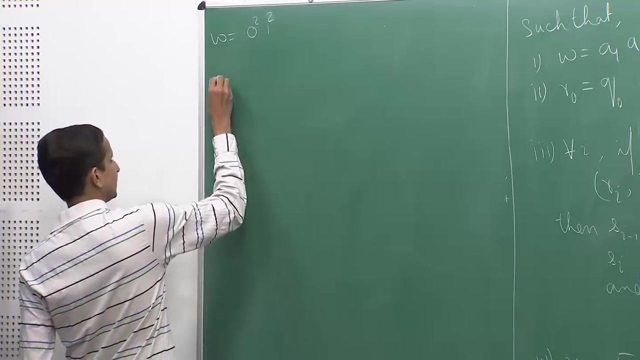 equal to a string 0,, 4, 0.. So that is principle 1, Scripture backwards: Why solבׄ타? 0 square, 1 square. So, on this string, what we will do is we will construct the following: 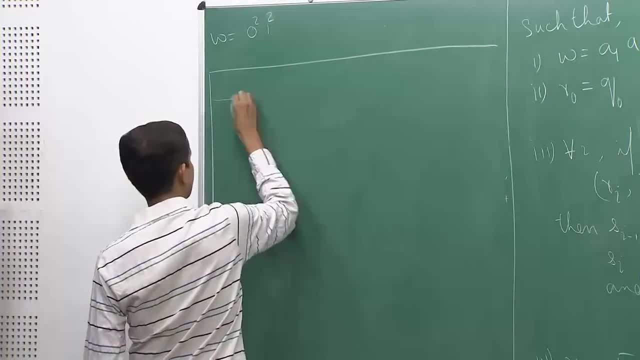 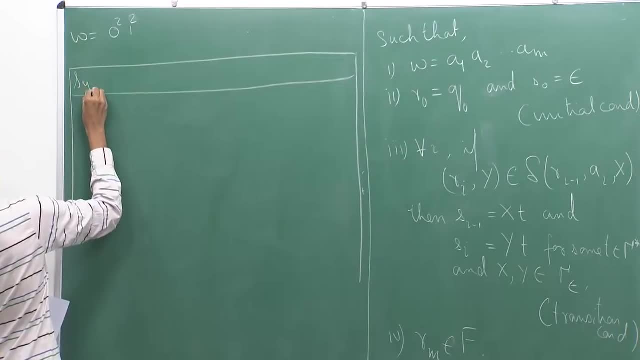 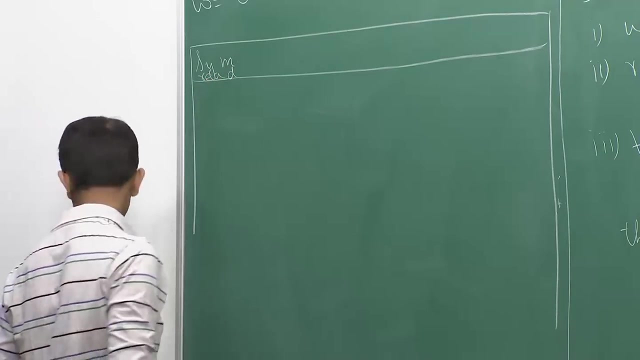 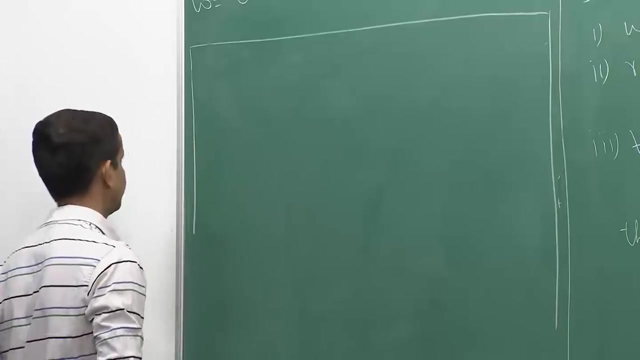 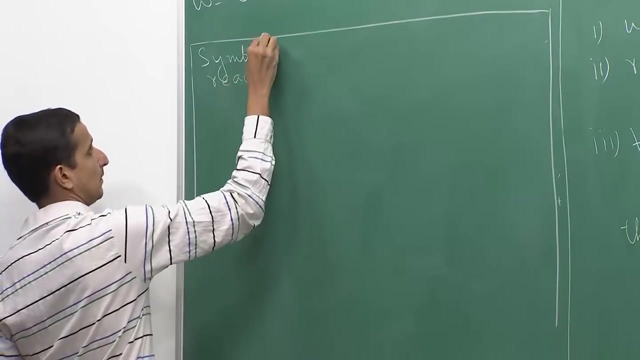 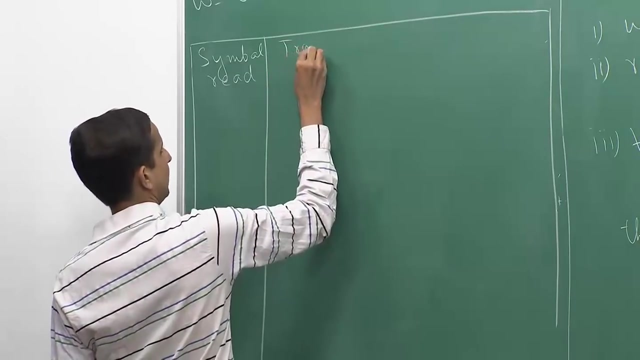 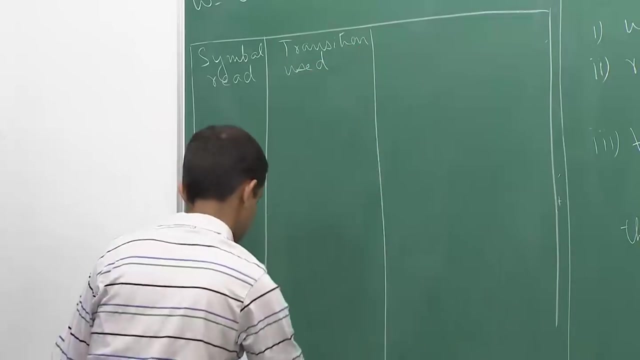 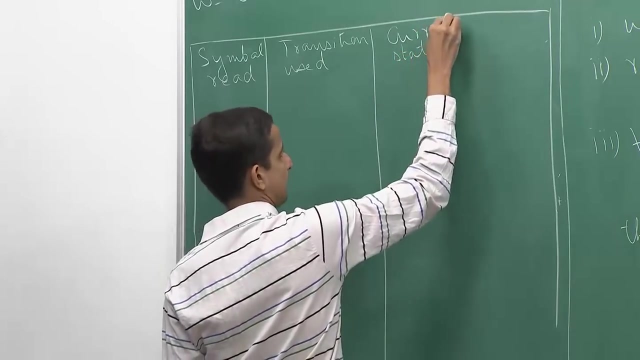 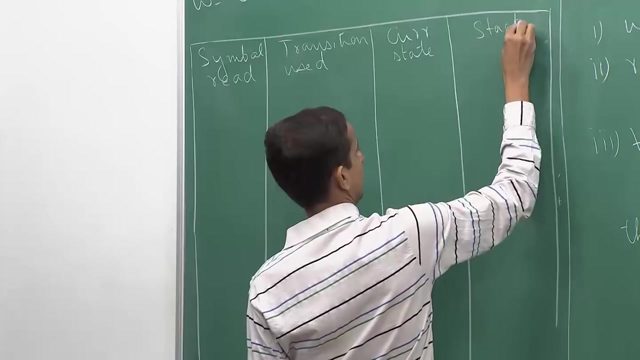 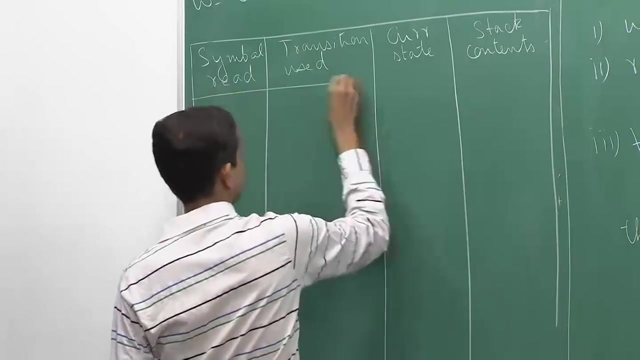 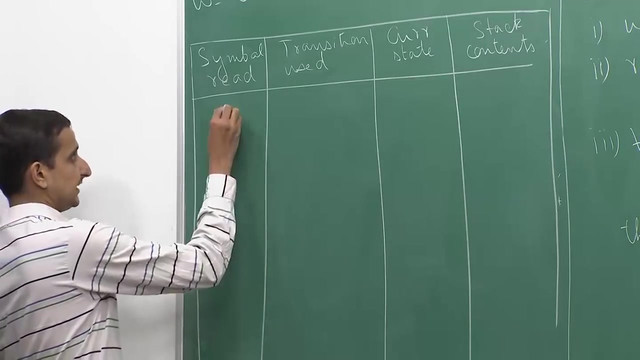 table where I have symbol red. I will just write it clearly. So I have symbol red, symbol green, then transition used, current state and stack contents. Okay, So these are the things that we will try to see. So initially, at the beginning, we 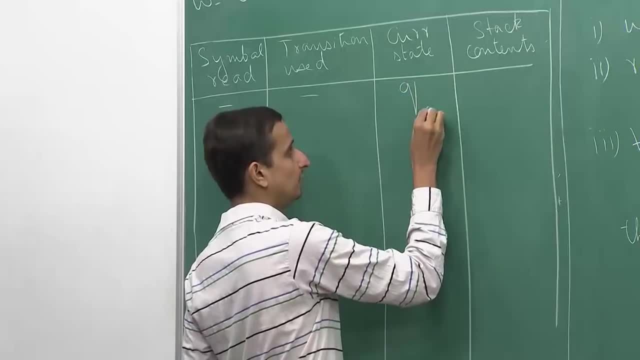 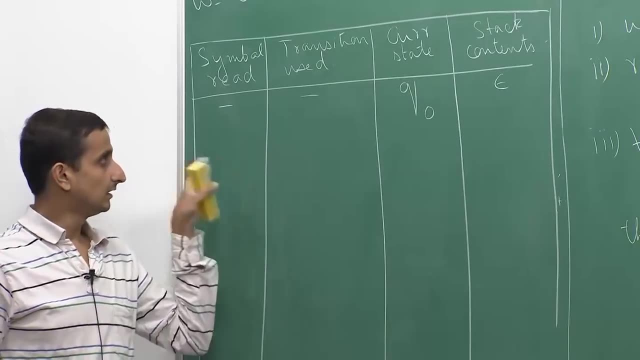 do not have anything. So the automaton is at the state q, 0 and the stack has nothing on it, So it is empty. So this is the initial condition. Now which symbol will it read? So first symbol will be 0.. So this is the initial condition. Now which symbol will? 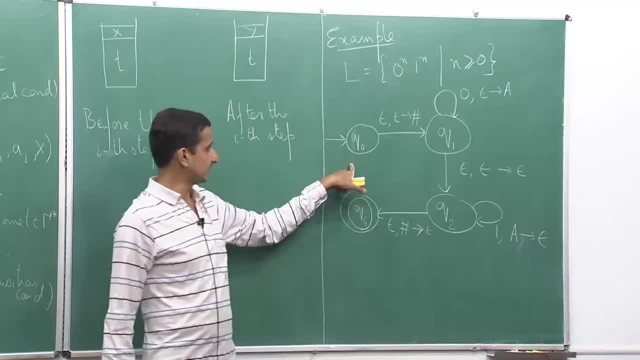 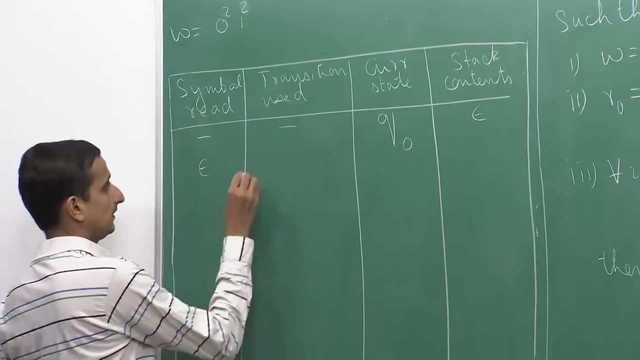 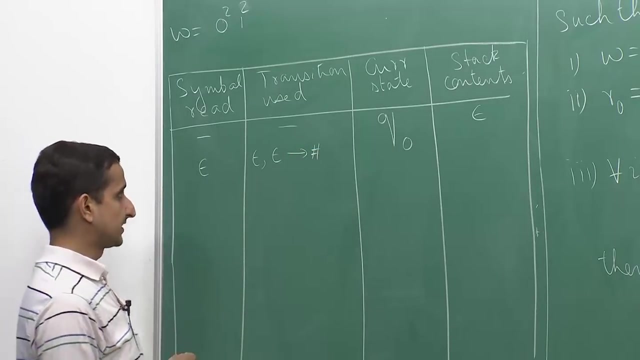 it read First. if you look at the automaton first, it has to go from q 0 to q 1, it reads nothing. So it reads the symbol epsilon. It uses the transition epsilon comma, epsilon to hash, It pushes in hash on to the stack and it goes to state q 1.. So now the stack. 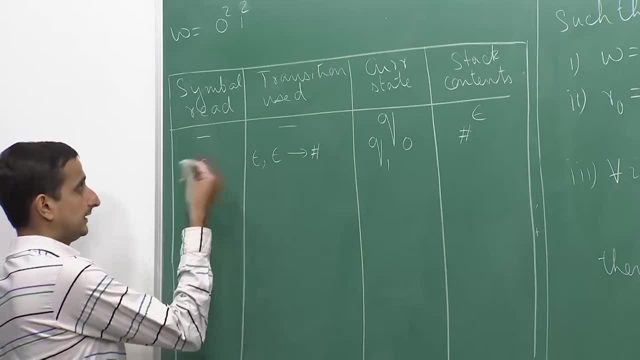 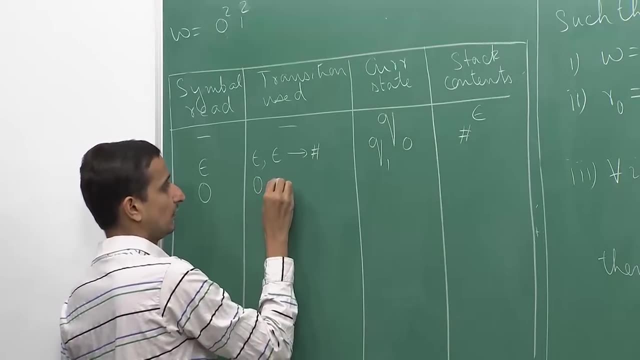 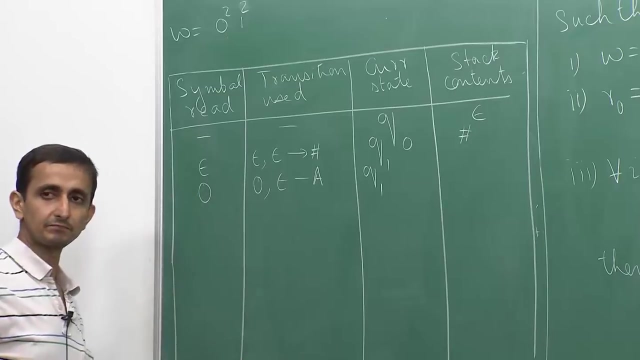 has hash on top. In the next step it is going to read the first, 0. So it will read 0.. Now you have it read. It will use the transition 0 epsilon to a. It stays at the state q 1.. 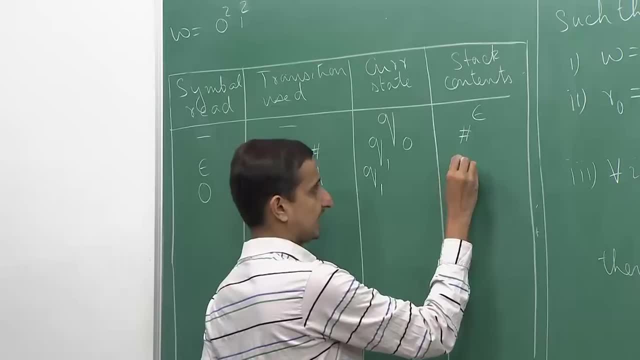 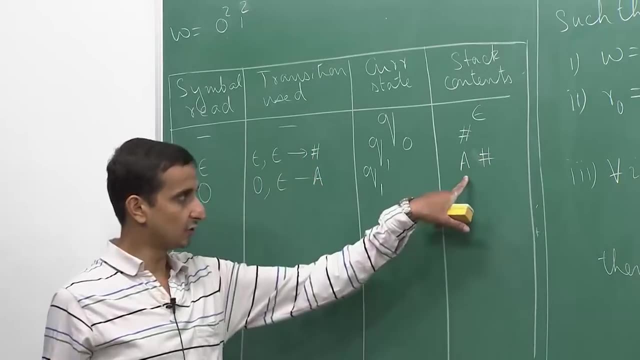 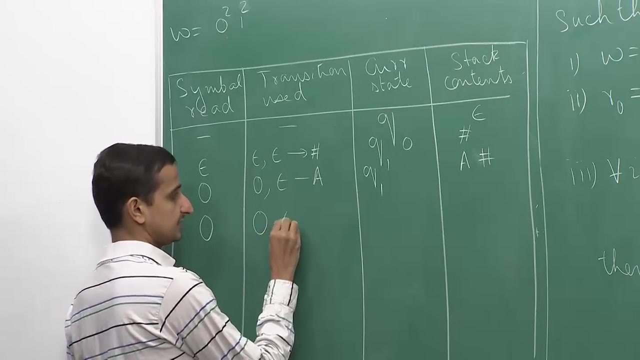 Okay, And now it has pushed a on to it. So now the stack has- if I just want to write it as a string, it has a hash a on top and hash below it. It reads the next: 0, sees: uses the transition again: epsilon going. 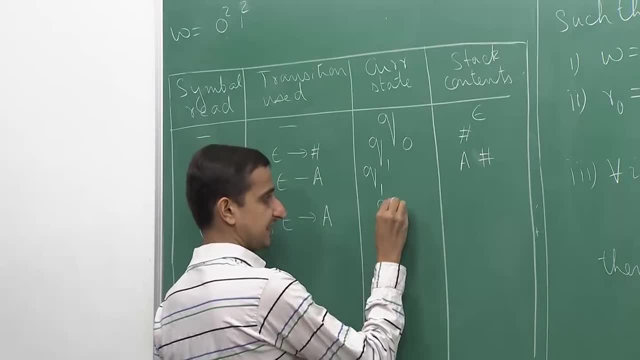 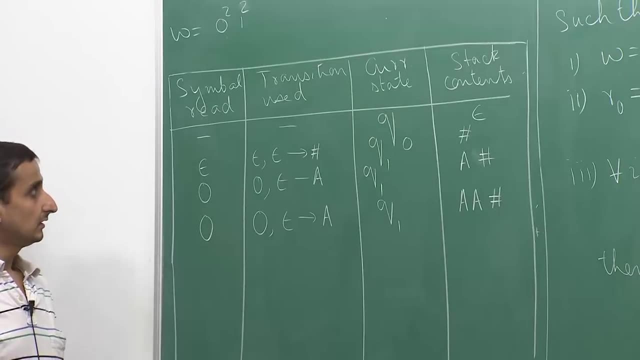 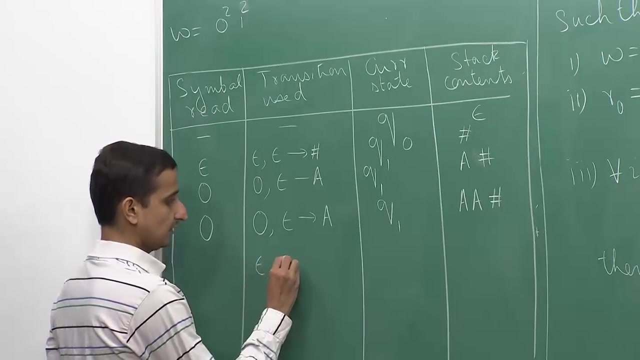 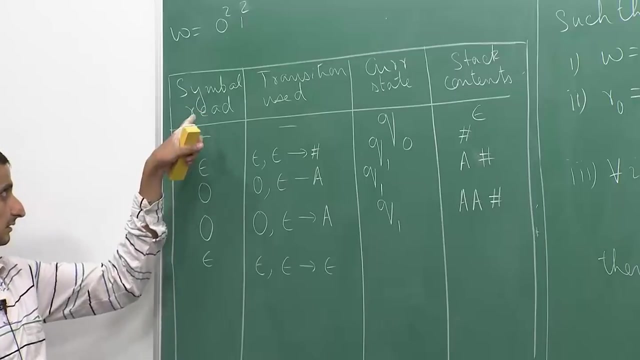 to a, stays at the state q 1, and now the stack has a, a hash. Now the zeros are exhausted. So now what we will do is that we will use the transition epsilon comma, epsilon going to epsilon. So we will not read any input bits, so the symbol read will be epsilon. 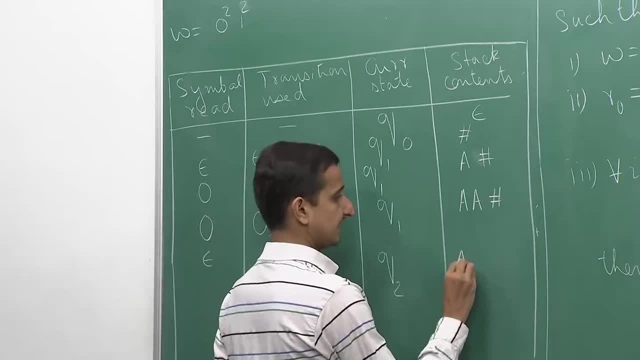 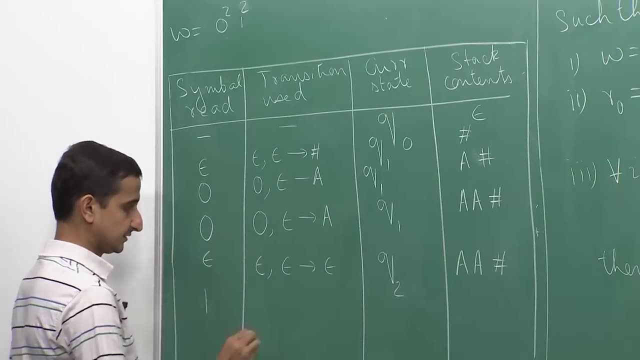 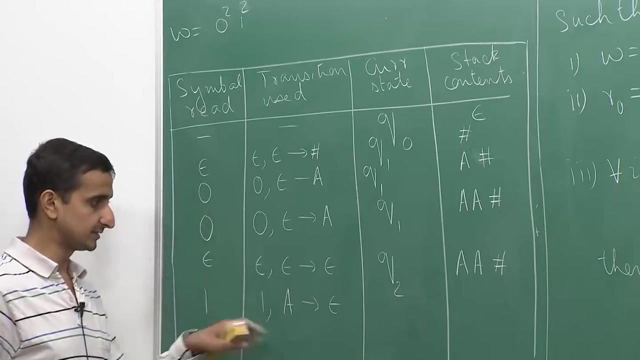 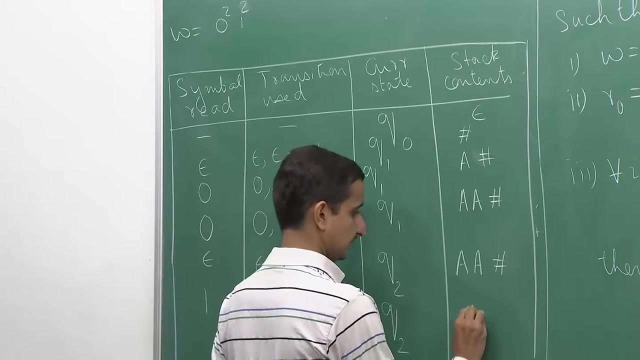 It moves to state q 2, the stack remains unchanged. In the next step it sees 1, it uses the transition 1 a to epsilon, which means that it is popping off a and it stays at state q 2.. So the current 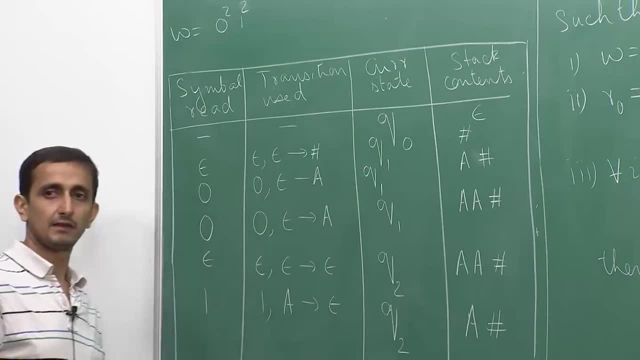 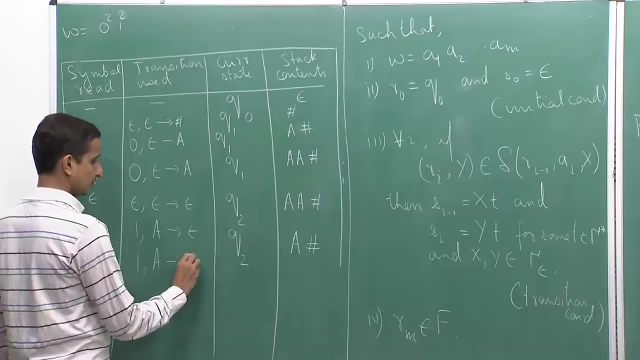 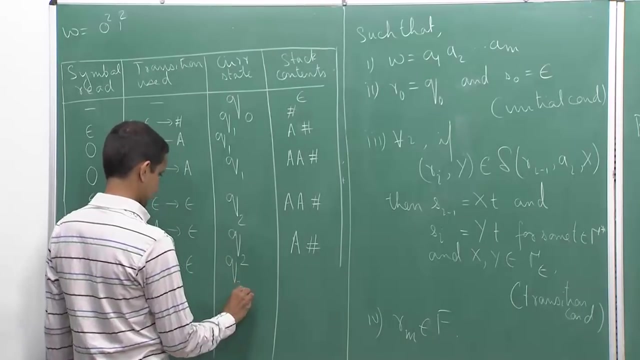 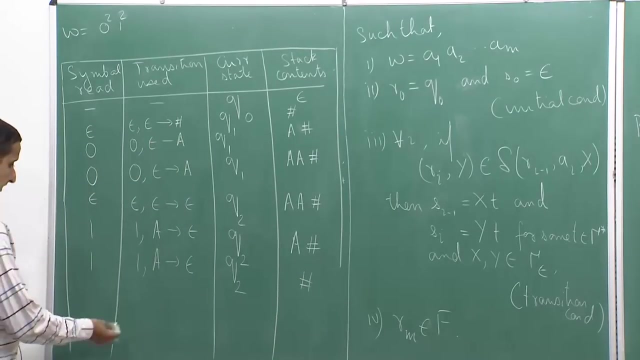 condition of the stack is a hash. Then it again reads a 1,. it uses the transition a going from a to epsilon and it stays at the state q 2.. Now the stack has hash on it, Now the 1s are read. now it can again without. 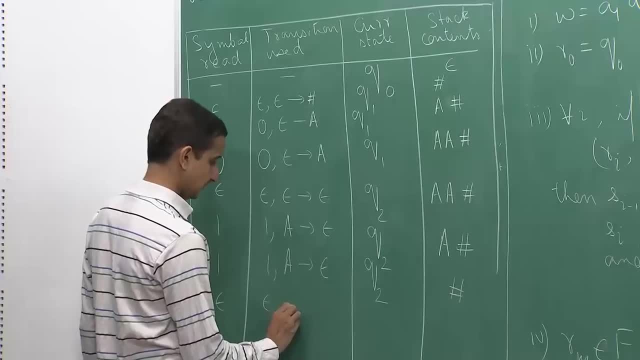 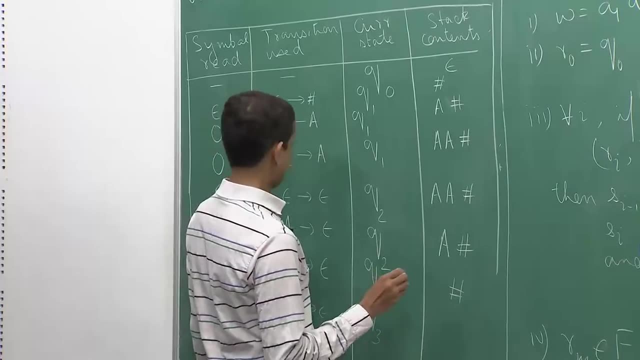 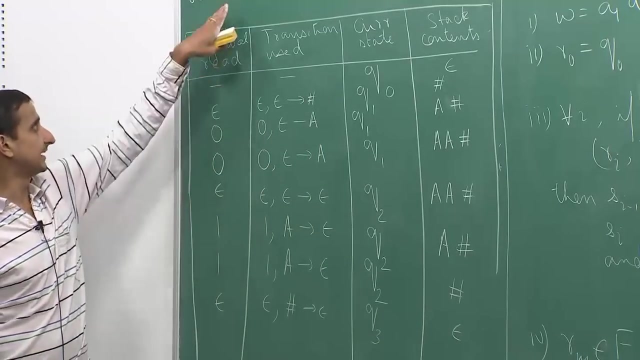 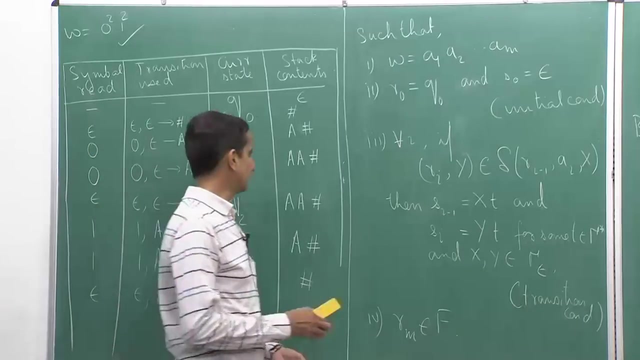 reading an input symbol. it can use the transition epsilon Hash going to epsilon, Move to epsilon, Okay, to the state q3 and basically accept. So now, if I concatenate all these, I get w, which is 0 star, 1 star, which means that this guy gets accepted. 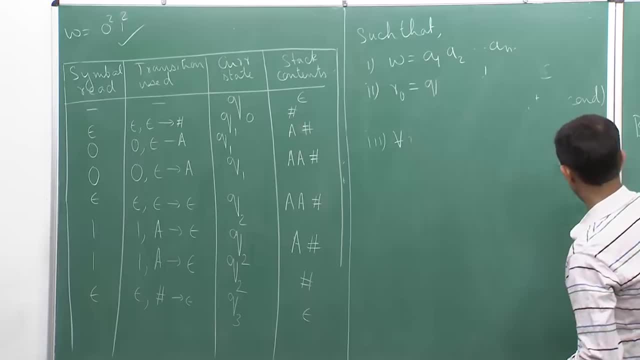 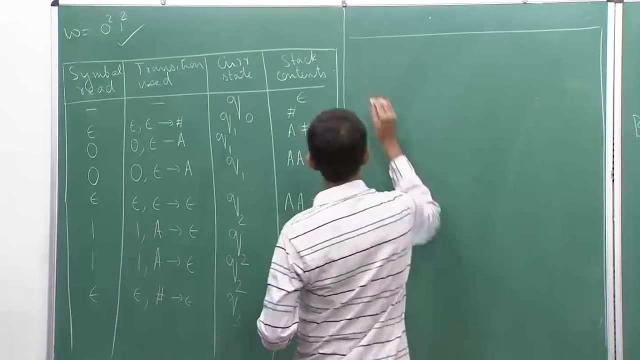 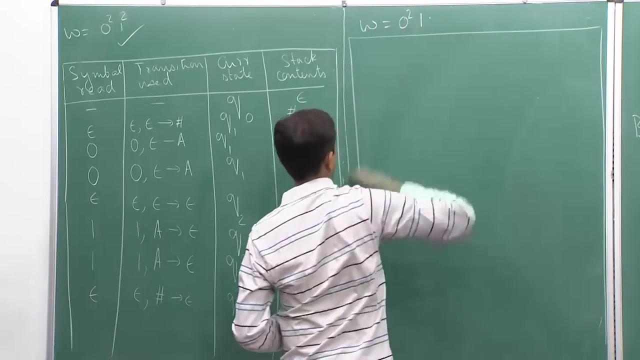 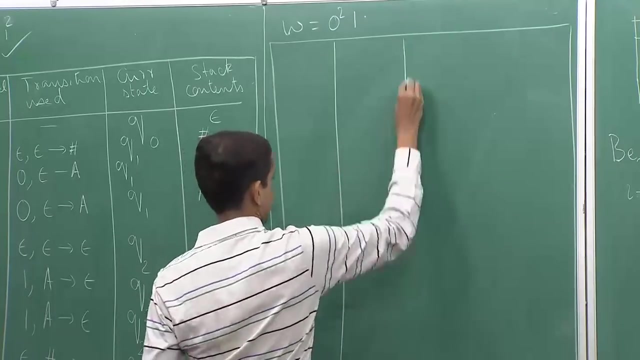 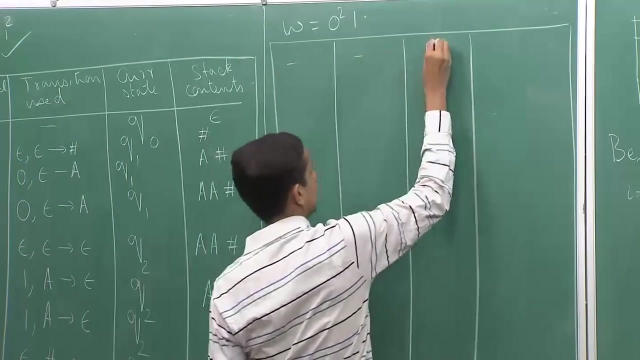 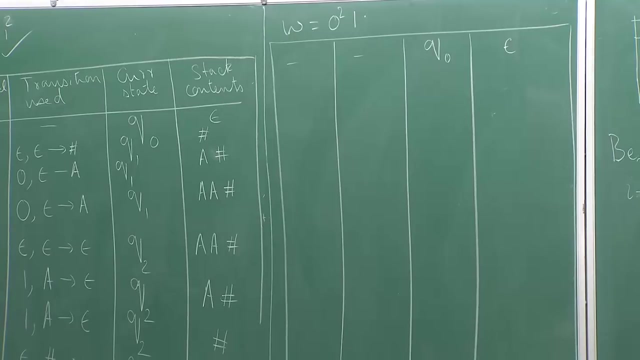 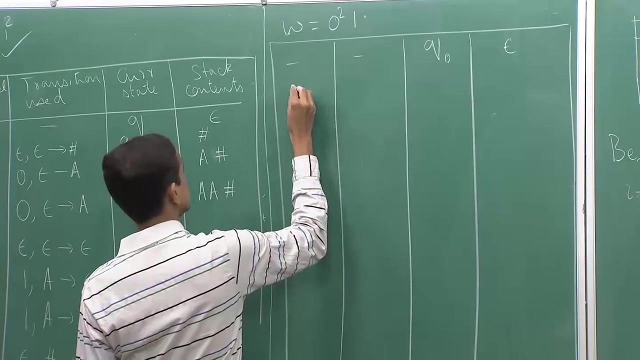 So now let us look at a similar table for a string which is not accepted, a string w which is 0 square 1.. Suppose, if I try to accept 0 square 1, what happens? So initially again, I have q naught and epsilon. On reading epsilon, I use the transition epsilon. 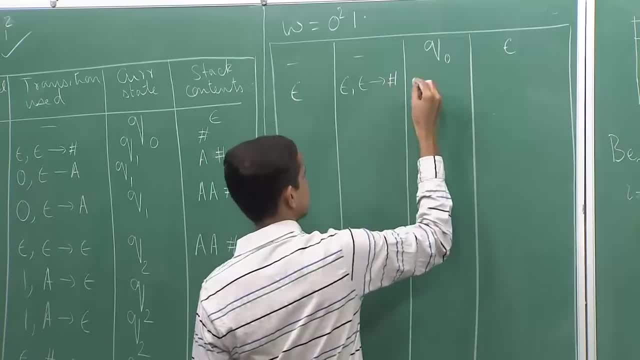 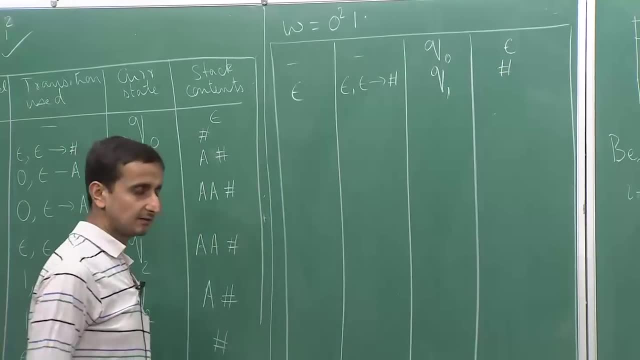 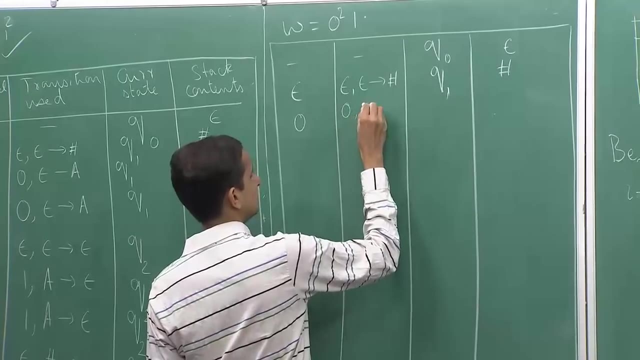 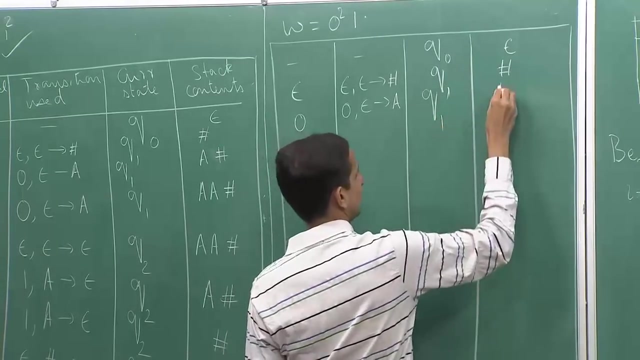 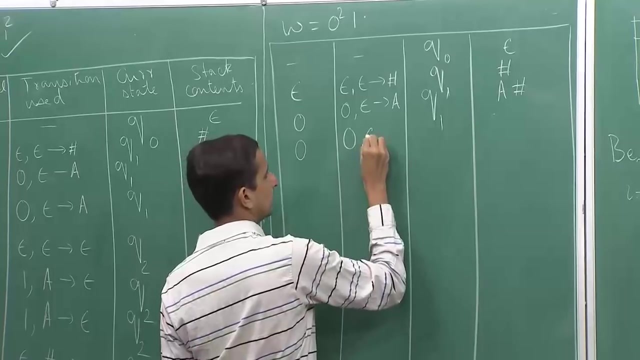 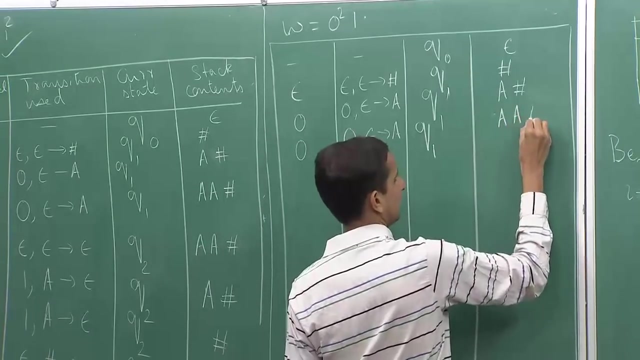 going from epsilon to hash and push, move to state q1. And push a hash onto the stack. Then, on reading 0, I use the transition 0, epsilon to a q1, a hash. Again I read 0. Again, I use this transition and go to a. 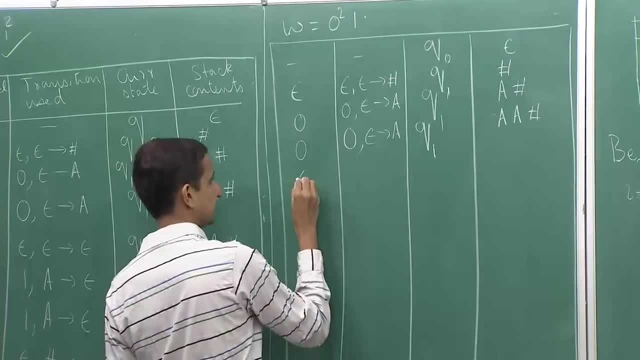 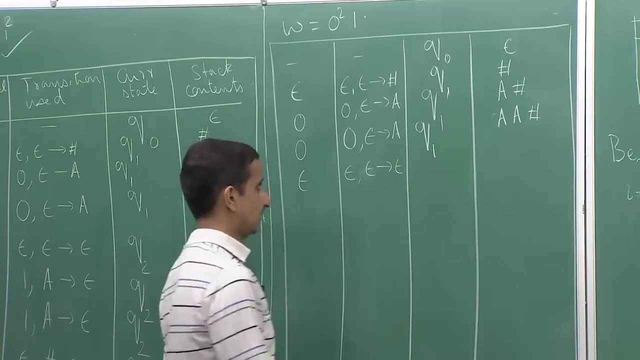 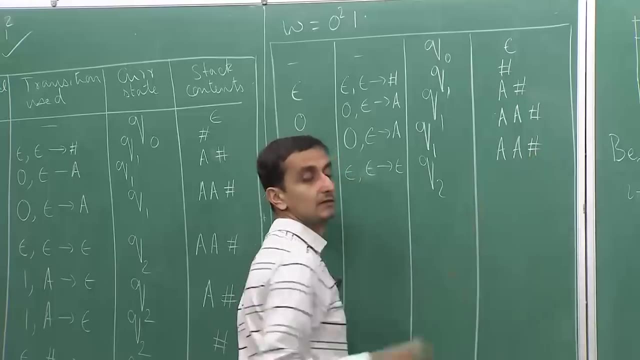 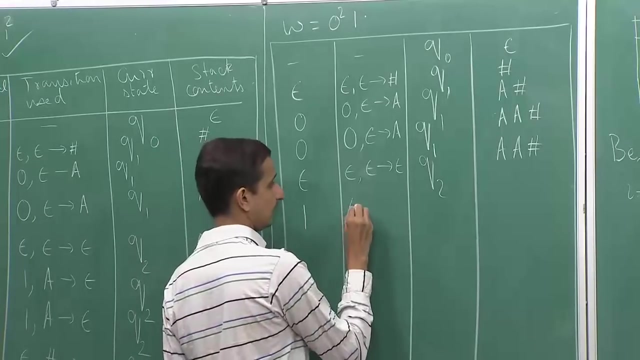 a a hash. Now I use the transition epsilon to epsilon, move to state q2.. Stack remains unchanged. Next I read a: 1. So it is 1, 0.. So it is 1, 0.. 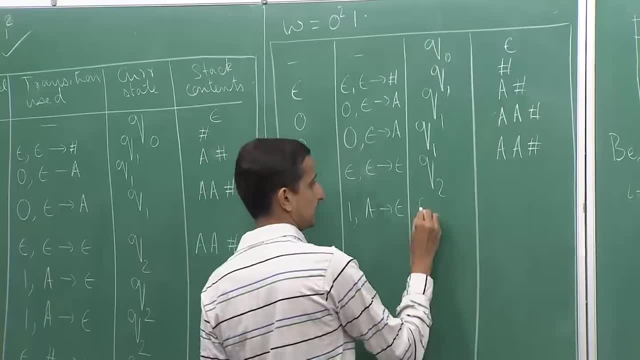 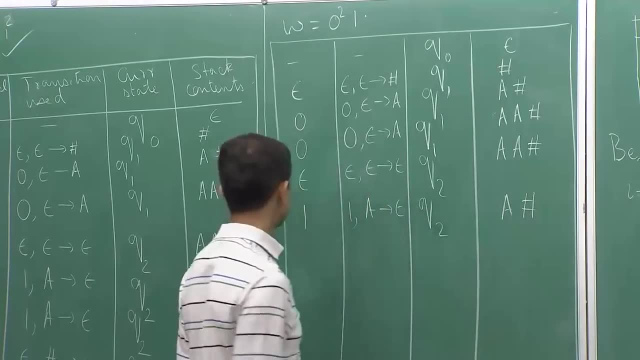 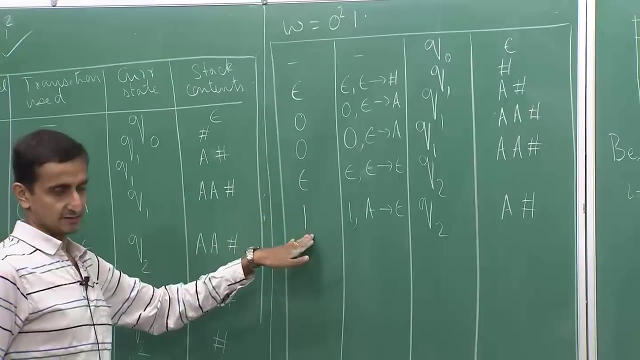 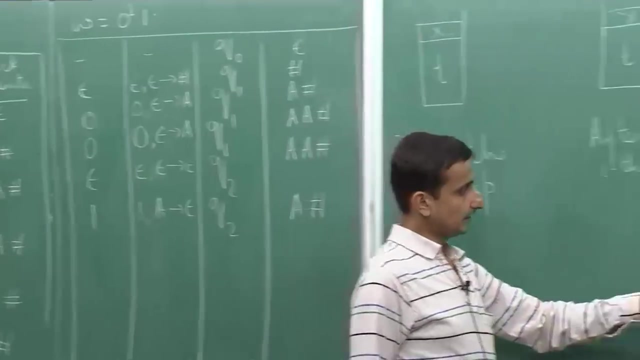 So a gets popped out, I remain at state q2. And the stack contains a hash. And here, at this step, my input is exhausted. I do not have any more bits to read, So I cannot use this transition to go to q4.. 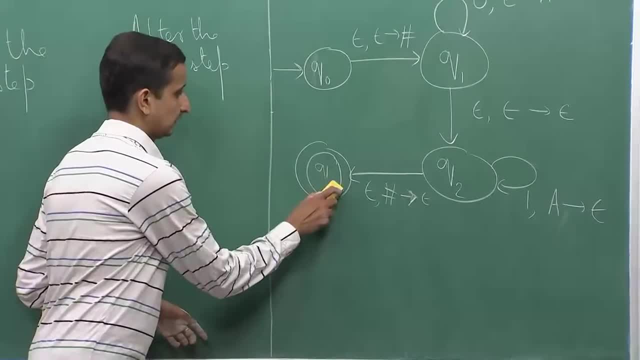 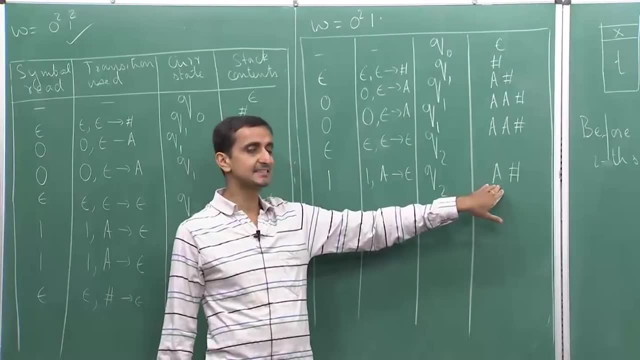 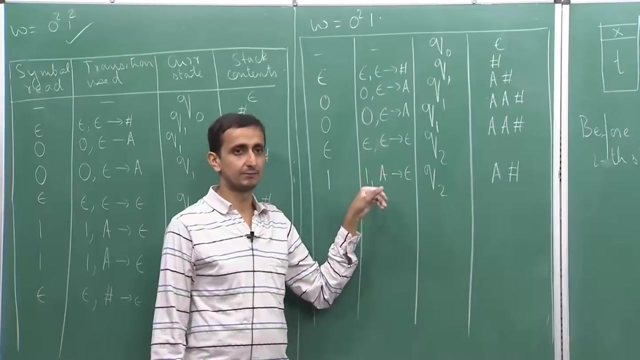 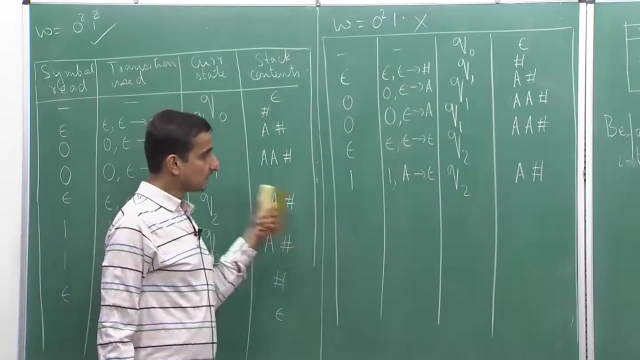 Q, so this should be Q3.. I cannot use that because now my top of the stack contains A, so I cannot use that transition. So I am stuck at the state Q2 and I cannot accept. So because of this, this string does not get accepted and it is non deterministic. So this is just. 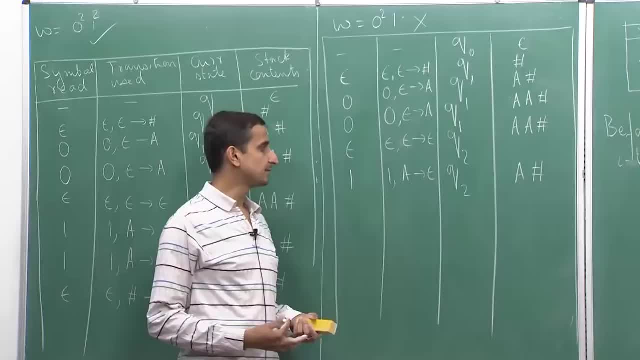 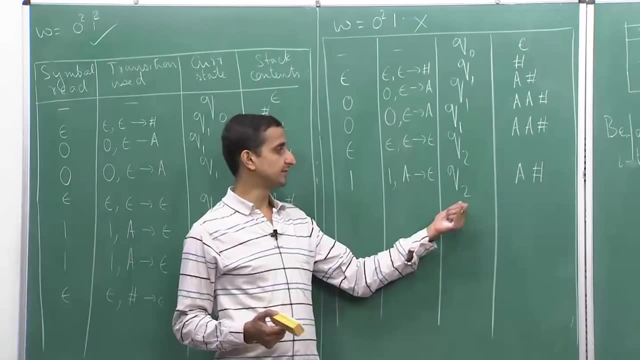 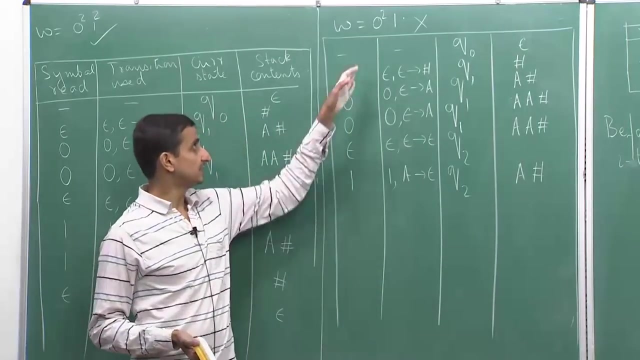 one computation path that I showed. You can also check that there may be other computation paths. you can try out other computation paths and you will be able to see that on none of the computation paths will you actually reach the accept state. Another example that you can try out is for the string 0, 1 square. For 0, 1 square: what?